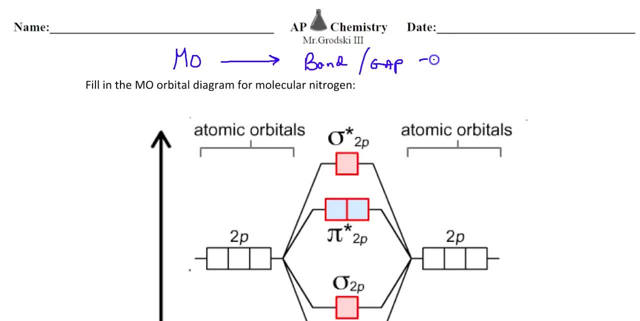 And then take you eventually to the idea of how transistors work. okay, Now transistors I'm not going to get to in this lecture, but I'm going to take you from the MO theory to the band or gap theory and then eventually to transistors. okay, 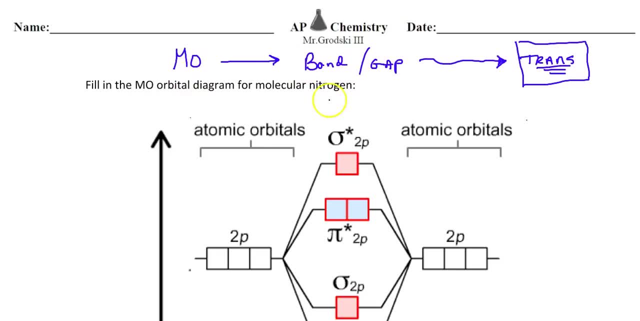 So I need to get through these two. So let's start Now. I did molecular nitrogen gas in class and we know through the valence shell theory that nitrogen is triple bonded. putting dots to a page or paper and then, of course, counting our valence electrons and sharing electrons: we need to get to an octet, okay. 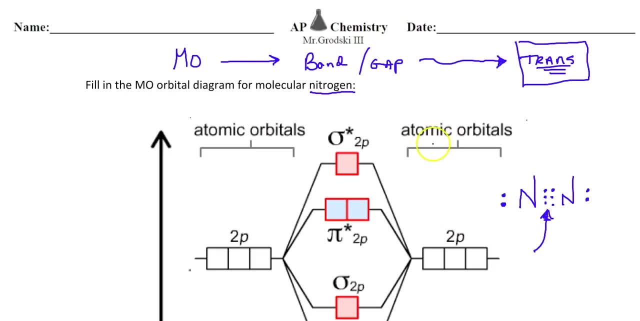 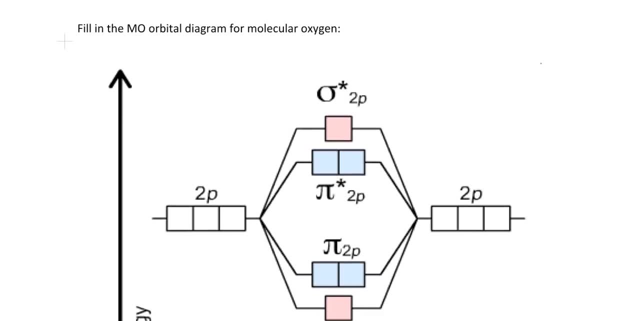 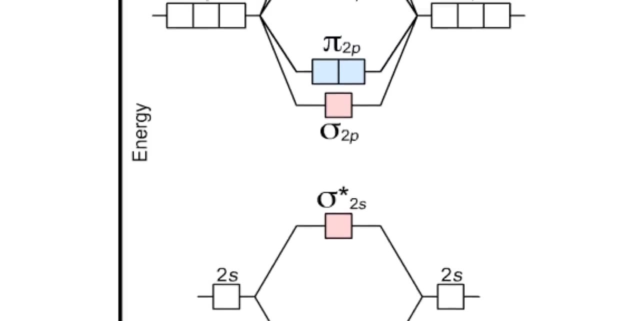 And when we do this for molecular nitrogen, we get the same thing. I want to get to oxygen, particularly Now. we did it in class, but for some of us it was too fast, Okay, Okay. so what we're looking at here, party people, is we're looking at an MO diagram and what we're going to do is we're going to put electrons from the two atoms coming together. 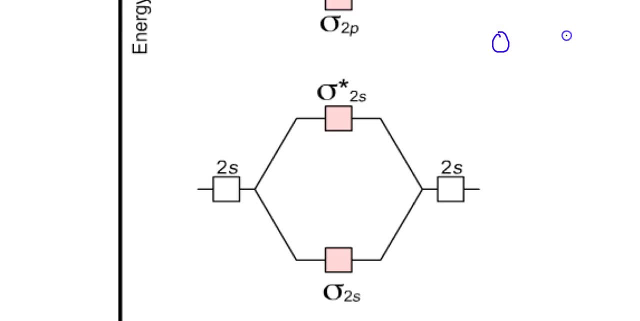 So again, think of, you know, an atom of oxygen, another atom of oxygen. They're going to collide, physically collide, and orbitals are going to interact. and when they interact, we're going to have bonding orbitals, which are more stable, and antibonding orbitals. 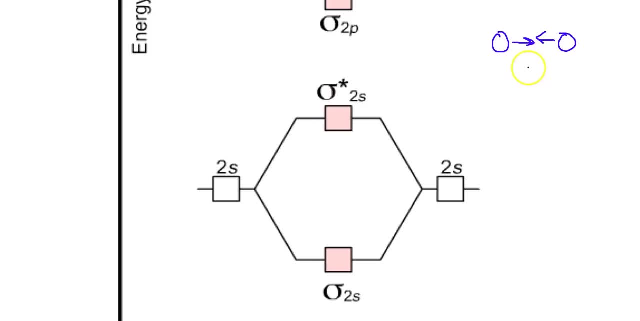 Remember this is not a valence bond theory. This is dealing electrons as waves and doing mathematical equations for the energy of these orbitals. when they constructively interfere- okay, which is a more stable scenario with electrons between two nuclei. and the scenario where they destructively interfere these waves- okay- and create electron densities outside the region between the nuclei. 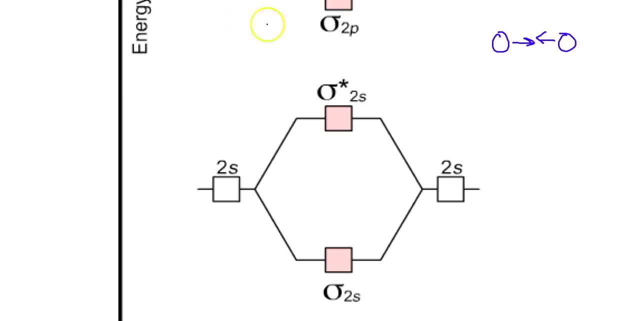 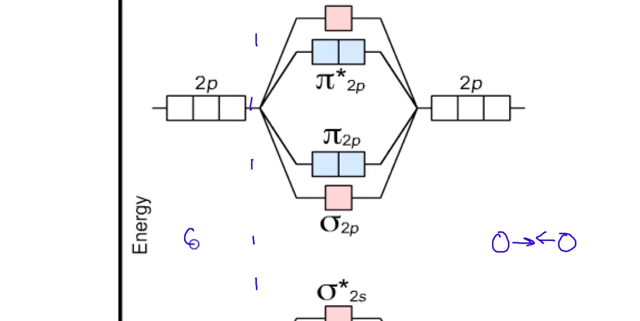 All right. so how do we start this? Well, consider- and it's very important you understand- that this part of the diagram is the atoms coming together. So if I scroll up, all right, I get the atoms on this side. So there's an oxygen on this side and its configuration is 1s2, 2s2, 2p4, and the oxygen over here. 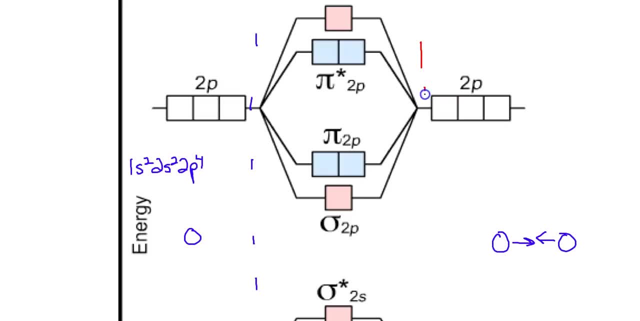 Okay, there's another oxygen that's coming together and that's the other oxygen here. okay, and it's 1s2, 2s2, 2p4 as well. So, real quickly, let's put the valence electrons in. All right, we can guess what's going to happen with the 1s2, as we did hydrogen today, but we have 2s2 here. 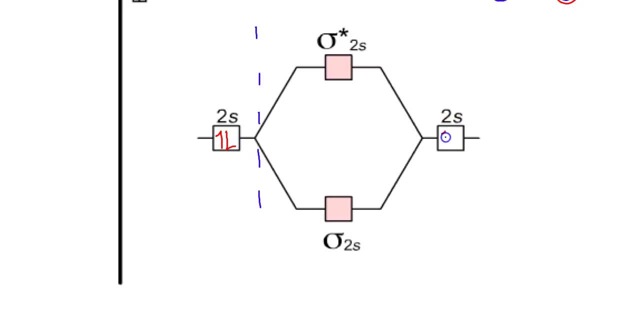 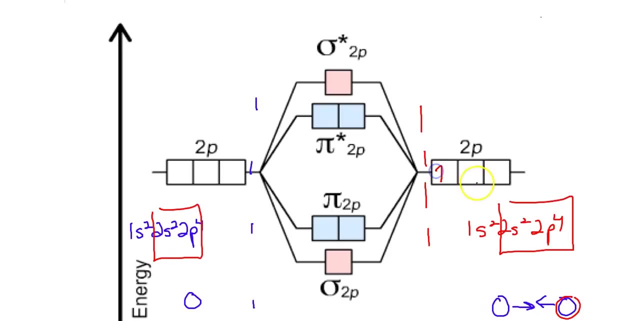 So 2s2,, I'm just putting the electrons in and then I'm 2p4.. Okay, so I'm going to put these in: 1,, 2,, 3,, HUD's rule 4,. I guess I should go blue here- 1,, 2,, 3, and 4, and I guess I should keep things the same. 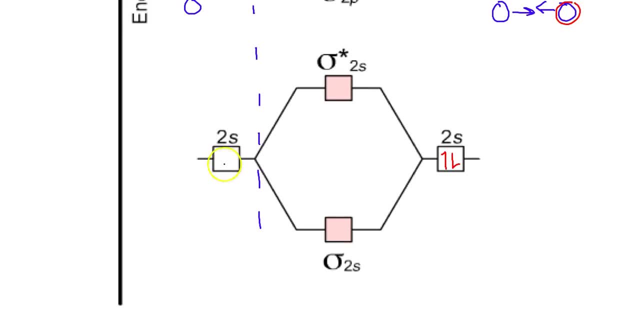 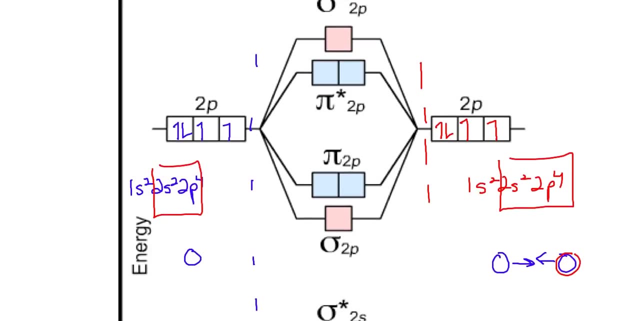 We'll do blue for the left oxygen. and I'm filling these orbitals, these 2s orbitals, because I have what? In the atomic orbitals? I have a fill. I have a filled orbital of S In the atomic orbital. I have 4 electrons in the P. 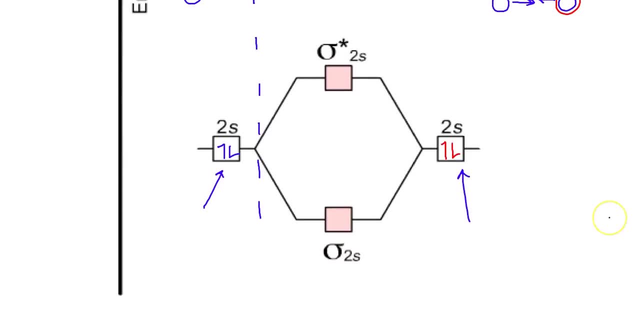 It's the same. Okay, so now what we're going to do is we're going to fill and talk about the two possibilities when these waves interact. Of course, the lower energy, more stable scenario is the sigma, and it's always going to be lower. 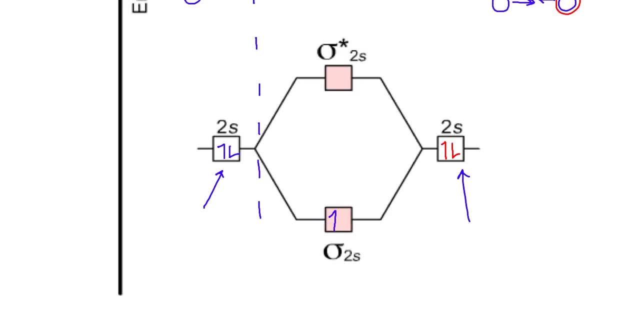 And of course I'm going to take one of these electrons, so we'll go up and take one of the reds and go up and down to show opposite spins. And so I've took half of these and now the other half. 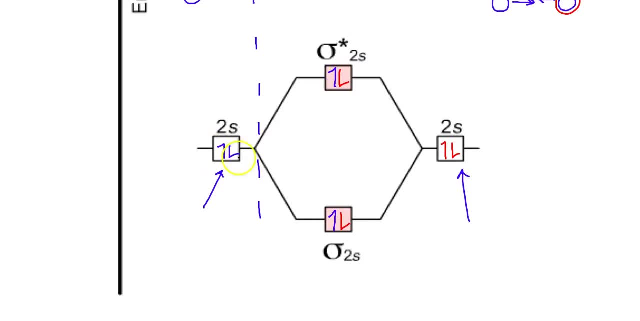 Go here, All right. so the two electrons in this left oxygen, one went to the bonding, one went to the antibonding and the opposite happened to the red oxygen. Remember, they're going to come together and their orbitals are going to interact and there's going to be constructive and destructive. 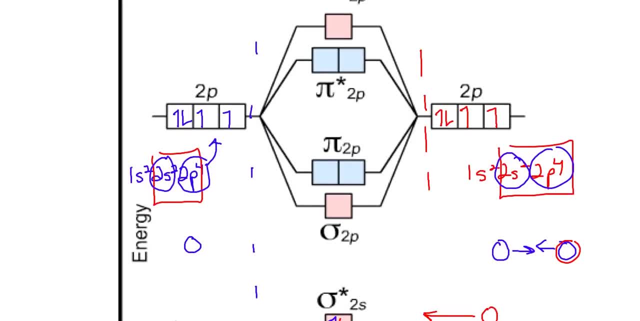 Okay, so we're almost done. Now we're going to take again these 4, so I've got 1.. Let's go down here And I'll take 3 of these showing opposite spins, And you notice I used 3.. 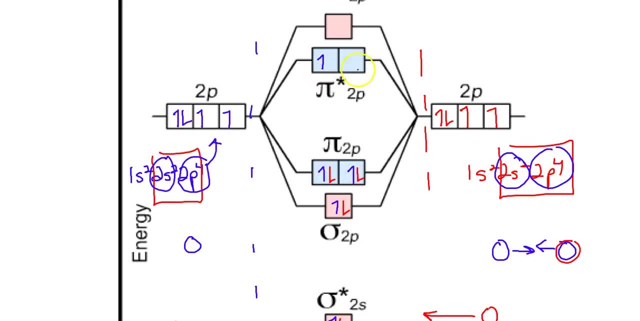 I need one more and same thing here, one more HUD's rule. So, if you notice, I had a total of 8 electrons in this 2P, total 8 electrons from both atoms coming together And I took 2,, 4,, 6 here. 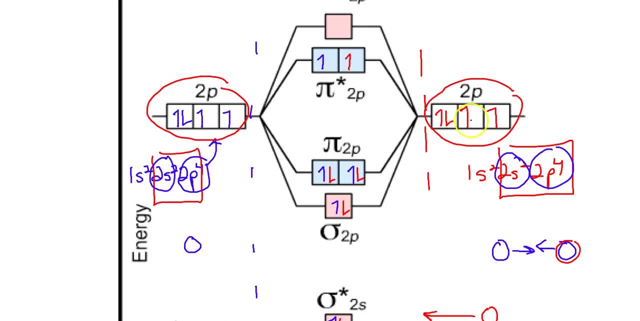 And then I have my 8.. So notice 4 of the blue, fill this way 4 of the red, And you notice we filled our bonding orbitals for a P. One is the sigma and the other is the pi. 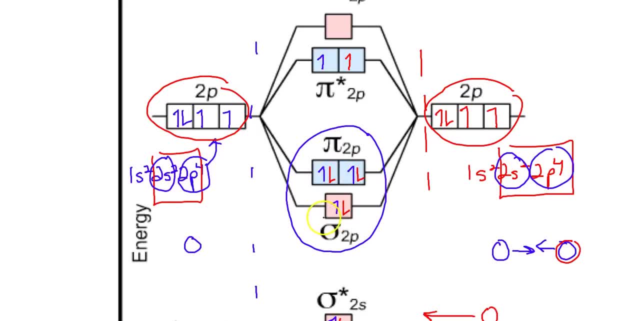 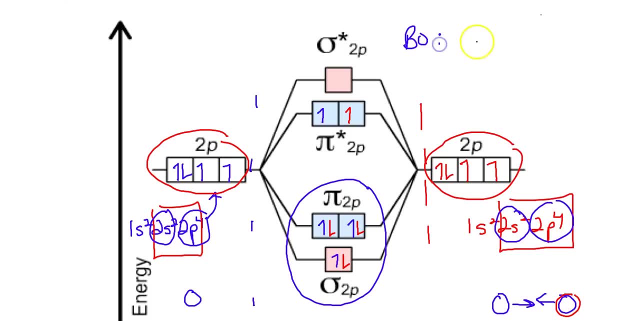 And you know the first bond is always the sigma, the second and third is the pi. Now, if you notice something, party people when we do bonding order. okay, bonding order is equal to the essentially the bonding electrons divided by 2, because a bond is a pair. 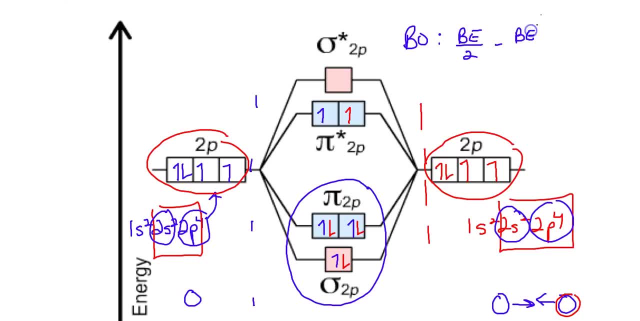 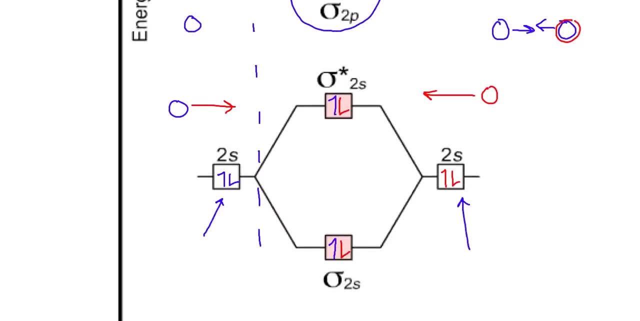 Minus the antibonding electrons. I'll do a little star here over 2, because a bond is a pair, And then notice how many bonding electrons do I have. I have? well, I have 2,, 4,, 6,, 8, who do we appreciate? 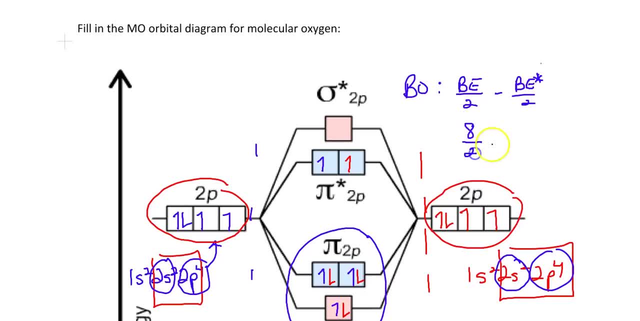 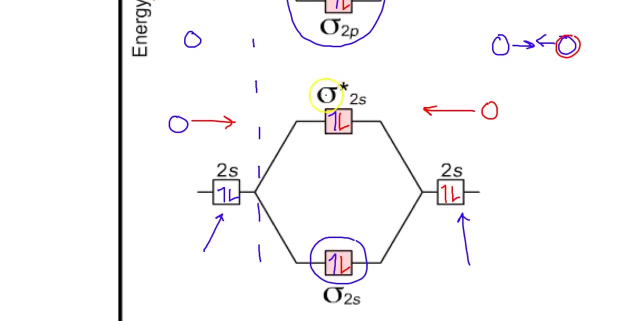 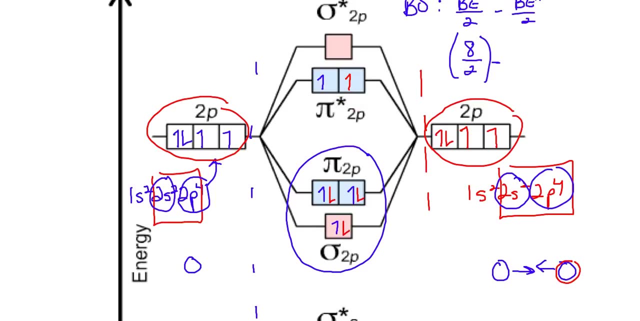 MO theory, of course 8 over 2, minus the antibonding. Well, we have 2 pi. I'm 2s star there, That's 2 there, And then we have this scenario the more unstable. So we have 4 altogether for antibonding electrons over 2.. 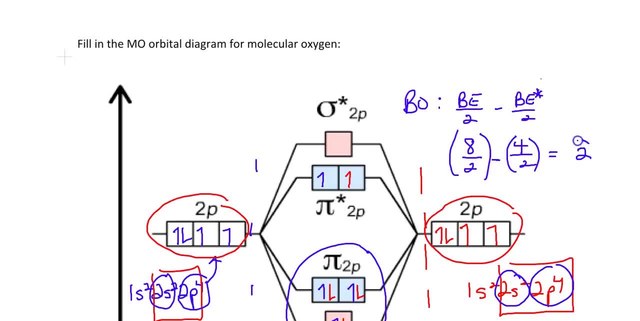 And you get 4 minus 2, and you get a bond order of 2.. And that speaks to the fact that oxygen has 2 bonds between its one region of 2.. All right, we know that from valence bond theory. 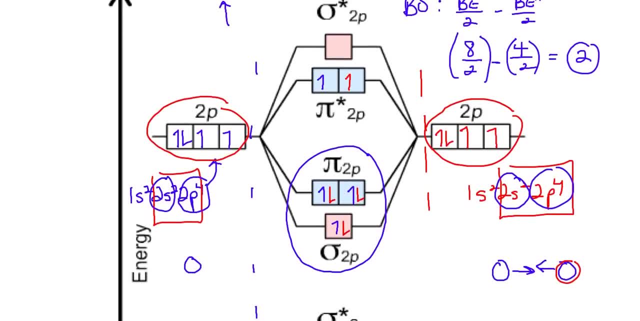 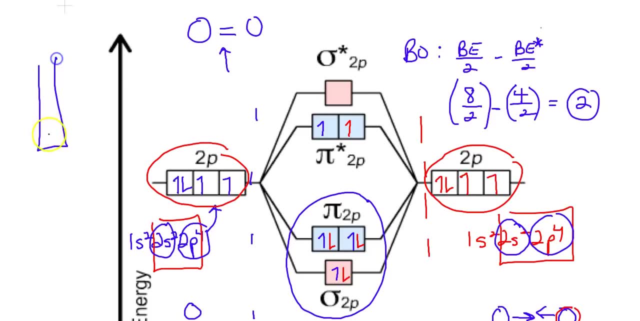 So what's the big deal? Well, the big deal is okay. we know from experience, From experimentation, that oxygen liquid is actually a little blue, lightly colored blue. And how can that be? Well, we can see from the MO theory that some of these electrons, if they're giving a color of light, 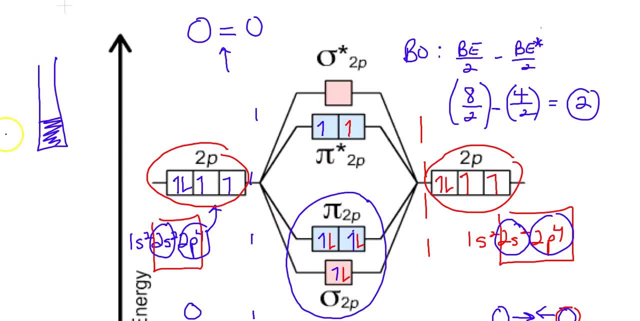 that means they're absorbing some wavelengths of light, right? So some light of all frequencies, of all photons of different frequencies are hitting, And then not all of it's coming out. You're seeing the blue come out because, well, maybe we're excited. 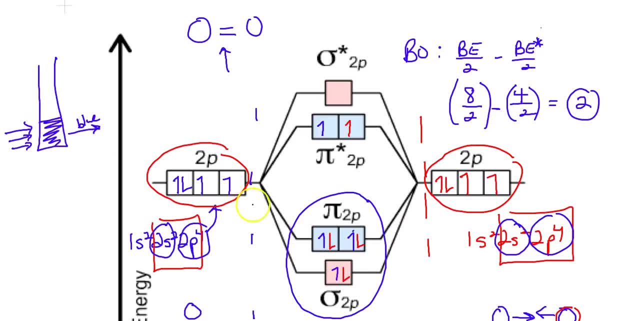 We're basically absorbing the yellow part of the spectrum, which means yellow photons, if I can do this, okay- are hitting this compound and giving these electrons energy to jump up. Okay, so they're absorbing that, All right, and so there's a gap being made between the bonding 2p orbitals. 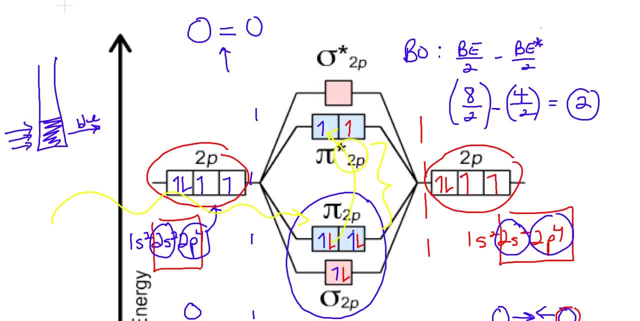 the pi 2p orbitals and the pi antibonding pi. So this gap really isn't big. It looks big in my drawing, but it's big enough that it can absorb a wavelength of light. or I should say small enough, because if it's too big okay. 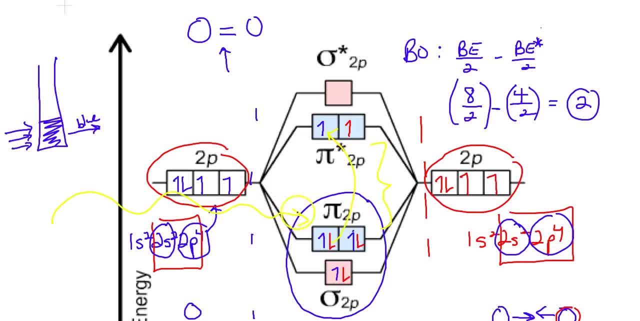 wavelengths of light which are tiny. okay, would be enough to move this. So the gap is small enough so that the wavelengths of visible light can be absorbed exactly. Remember, to get from one position to another is an exact amount because it's a quantized effect. 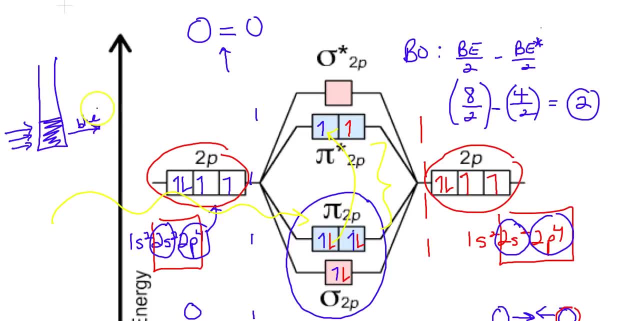 The atom is quantized, So the color Given off is the idea that we have this little gap. Remember, I talked about the fact that MO theory leads us to something called gap theory or band theory, And again what's happening is we're creating a little gap here for oxygen that we would never 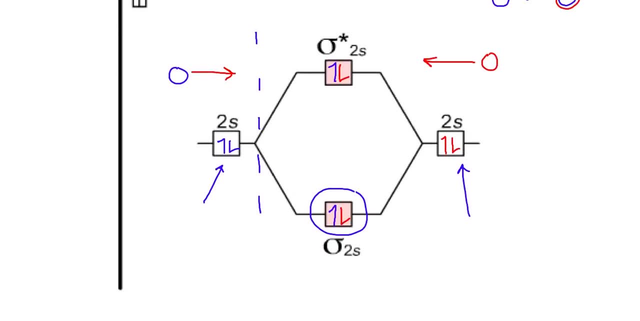 ever consider if we didn't use this theory? And you say, well, why, Mr Grodzki? Well, if you take oxygen and it's six valence electrons and we put it with another red oxygen and we use it for oxygen, we get a little gap. 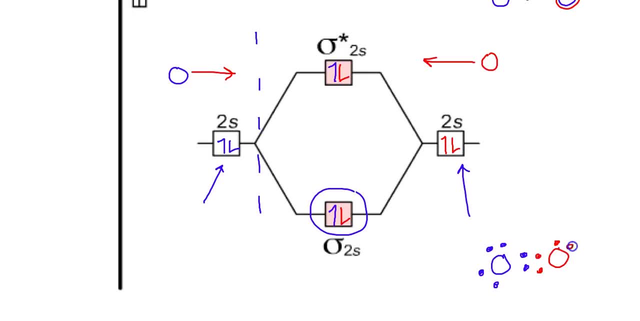 We use valence bond theory, What we're going to get is what we expect. the double bond- Remember every what Oxygen, by having a double bond, feels like it has its eight. there It's the valence shell that we talk about. 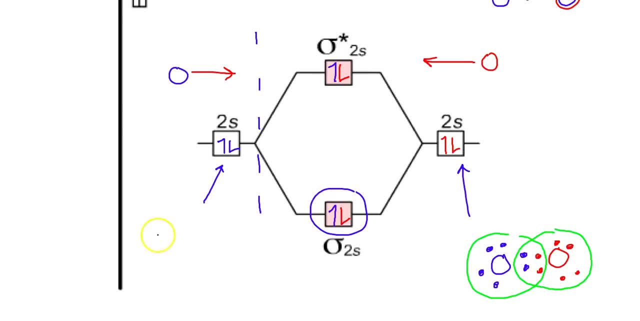 So this is expected, If you think about oxygen, as we did here. this blue one is what? 1s2, 2s2, 2p4.. What does that 2p4 mean? Well, that 2p4 means that we have four electrons in our 2p orbital. 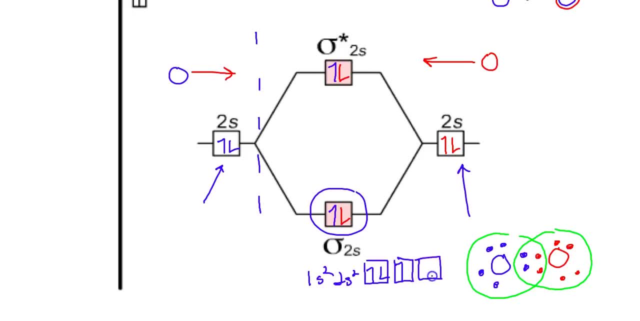 I know I drew this before, but I need to make this point. And then we have a red one, 1s2,, 2s2, and also 2p4. And we still have four. And so what happens, party people, is we're going to have what? 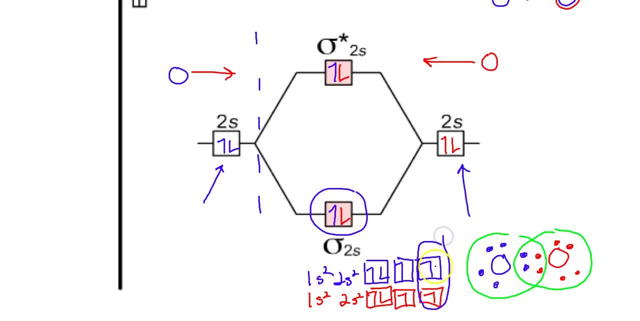 A sigma bond with one of the p's, And by them doing what But overlapping? they feel like they have two, And so this probably is one of these is a sigma bond, can't know for sure, And the other one is the pi bond. 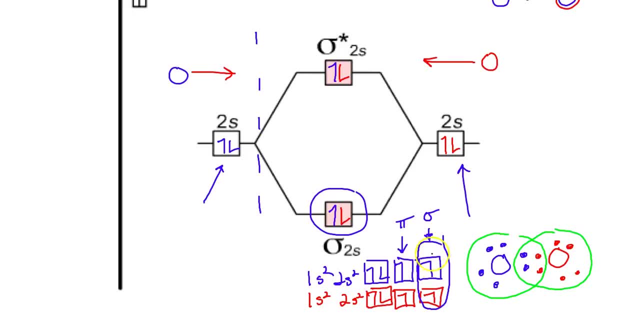 So you can see that unhybridized p orbitals basically either overlap directly or indirectly overlap with the pi bond to make them both feel like they have filled p orbitals. And that's the valence bond theory. So when these guys overlap, this guy feels like there's another one. 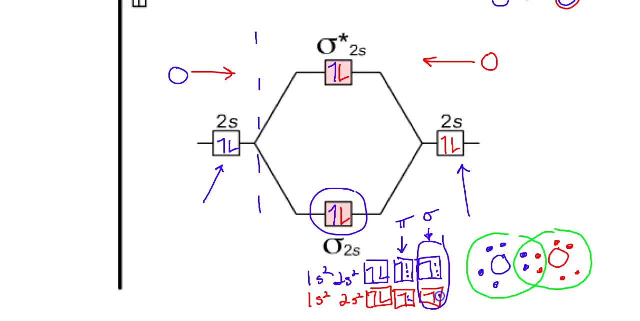 And this one feels like this And they all feel like they have another one, which means: where is the what, Where is the lone pairs, If every single oxygen in this setup here feels like they have the octet, which means what They're: 2s2,, 2p6 by sharing okay? 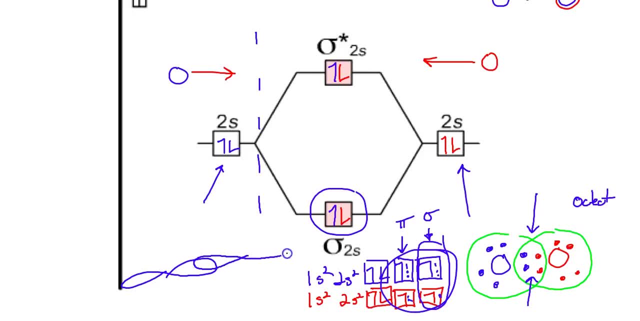 Remember that p orbital overlapping another p orbital to feel like they both have what, Two and the same thing with the what, The other p orbital giving us the pi bond. right, This is the sigma and this is the pi Why I'm drawing it off to the side, not really sure. 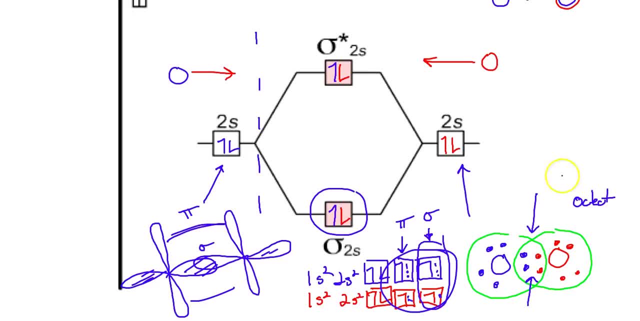 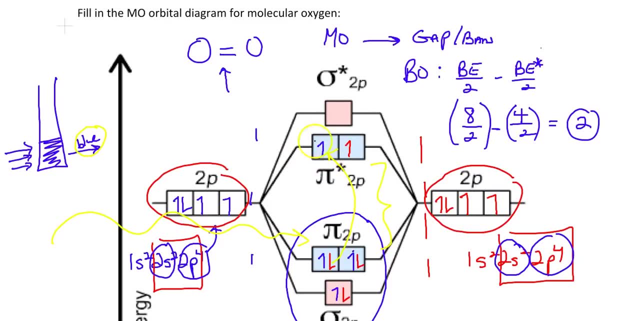 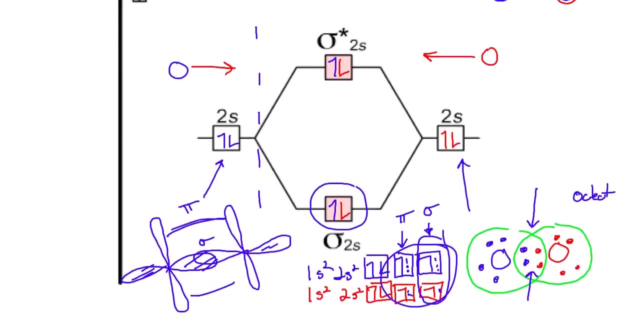 I guess I'm being artsy. So they both feel like they're filled. So where do we get singlets or occupied unfilled orbitals here? We don't in this theory. So valence shell theory does not predict that oxygen would absorb wave-like 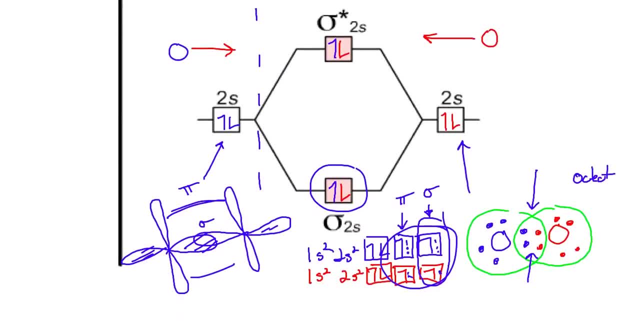 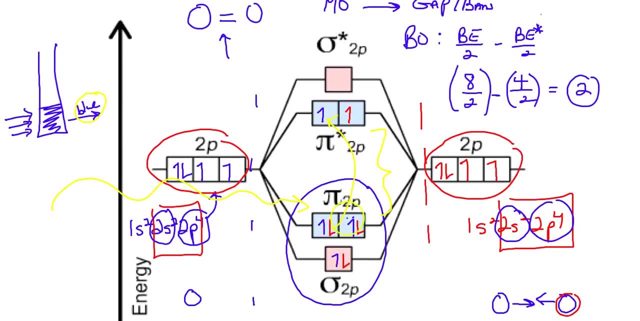 wavelengths of light because all of its orbitals are filled in the valence bond theory when they bond to get this octet, Whereas in molecular MO theory, more advanced theory, this shows us that there are okay unpaired electrons in these anti-bonding orbitals that give the ability to absorb wavelengths. 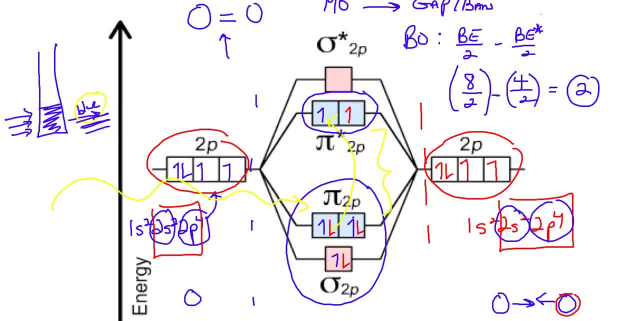 of light. More importantly, though, as I will show you in class, okay, this determines the idea that oxygen molecules are what Paramagnetic? Remember we talked about this? having lone pairs means you do not have another electron in this orbital of opposite spin to cancel out this spin. 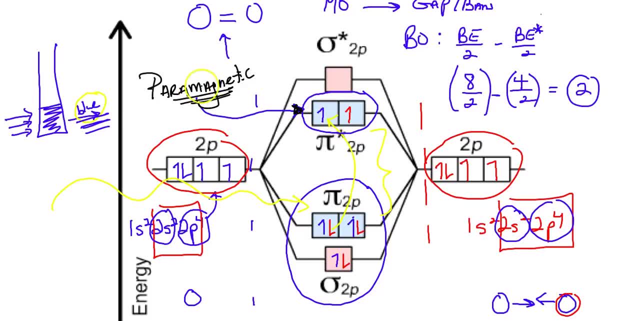 So these spins will go together, creating a paramagnetic ability, meaning that they are affected by a magnetic field. Okay, which I will show you with the liquid oxygen demo. This is the liquid oxygen demo that I have taped or have a video for. 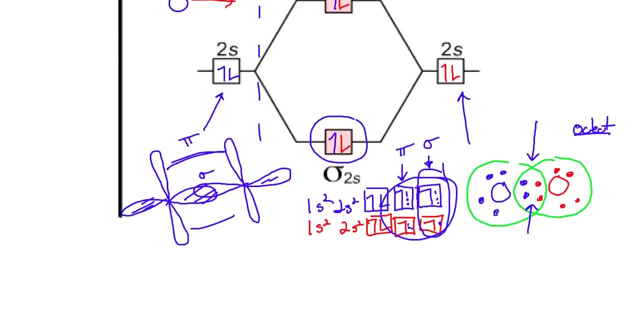 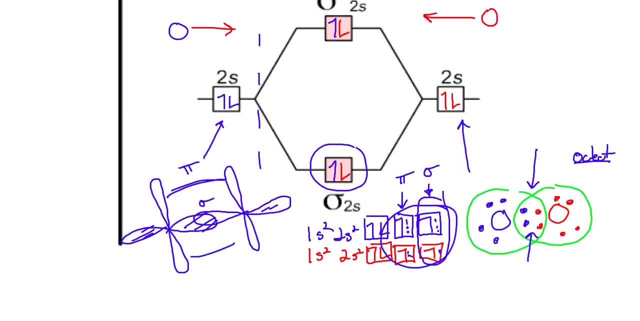 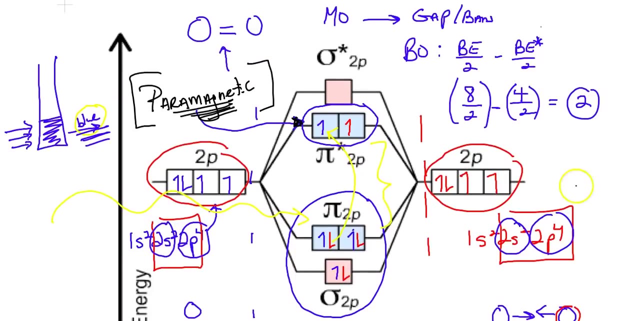 Pretty cool. And again, that's only shown with MO, not with valence bond theory. So the MO theory gives us more information or fills in the gaps, so to speak. no pun intended, All right. So in this case, in this diagram here: okay, the MO created this kind of ability to have. 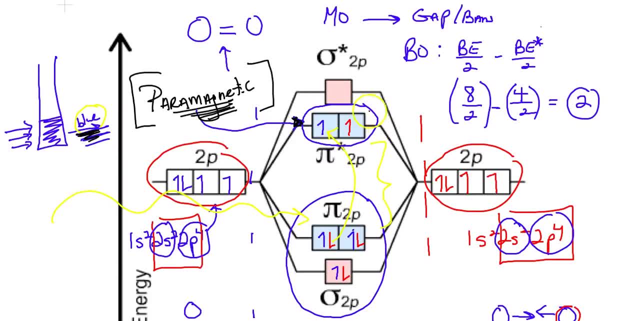 a gap to create a blue color and gave us these lone pairs, Okay, So that we can basically understand that and explain, or at least demonstrate through this theory, the paramagnetic ability of oxygen that otherwise would not be. So where do we go from this? 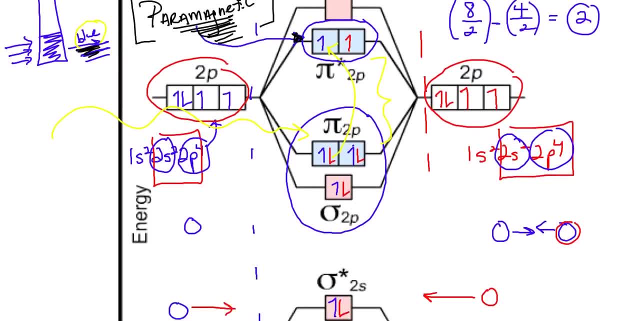 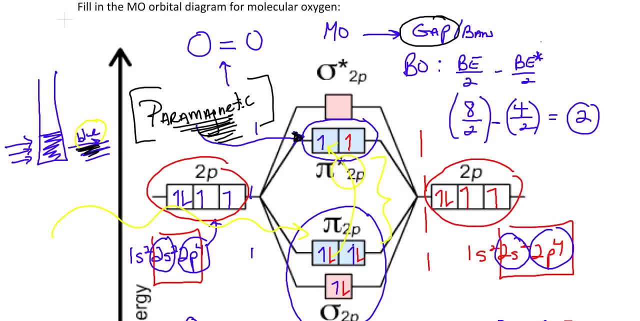 Well, understanding this opens the door for something called gap theory. Okay, Now I know. we said that this idea of having anti-bonding orbitals, in this case, allowed for us to understand this, For us to understand a gap that was created. 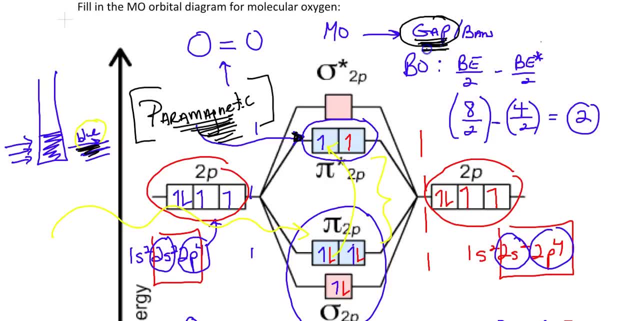 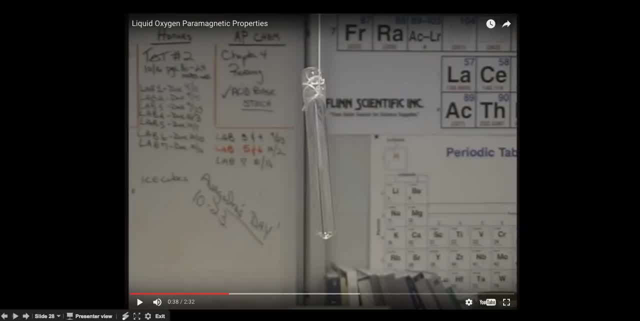 But there's more to it in gap theory, but it's based upon- I should say on MO diagrams, So let's get to it. So here I have a tube hanging in the class and I'm going to add some liquid oxygen. 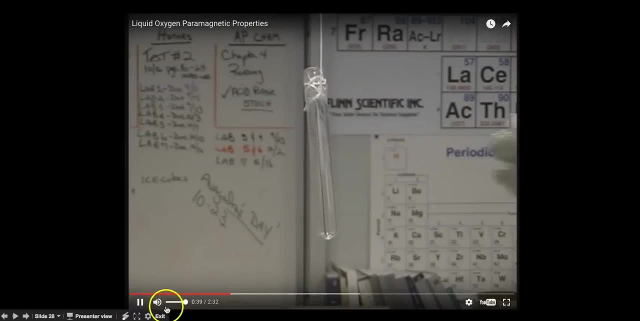 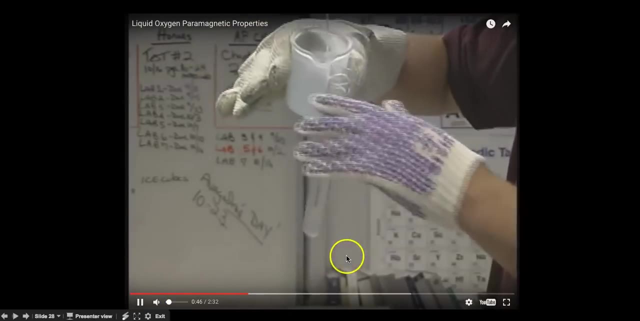 Look at the color: It's a slight blue, Okay, So I'm going to add some of that. It's about 183 degrees Celsius, Okay, And that's tough to see, But it is a slight blue. It's not, like you know, royal blue. 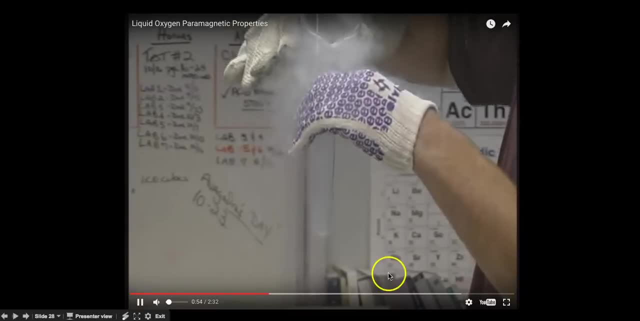 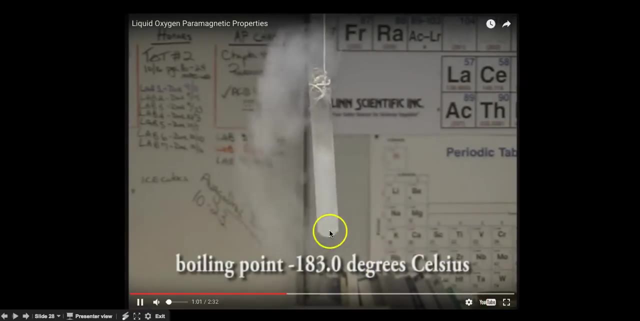 And what happens is, of course, you get frost on the outside, So it's hard to see it sometimes, But it is a slight blue hue And I make it with liquid nitrogen. So in any case, what's really cool is because of that lone pair of electrons predicted by 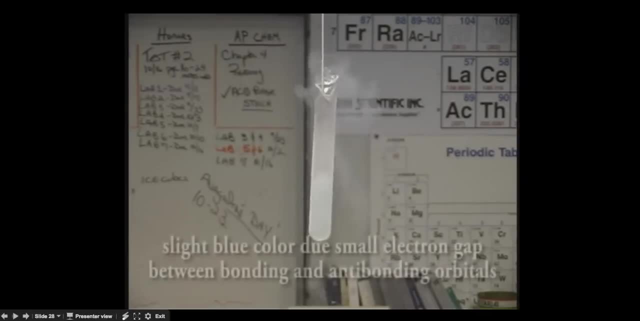 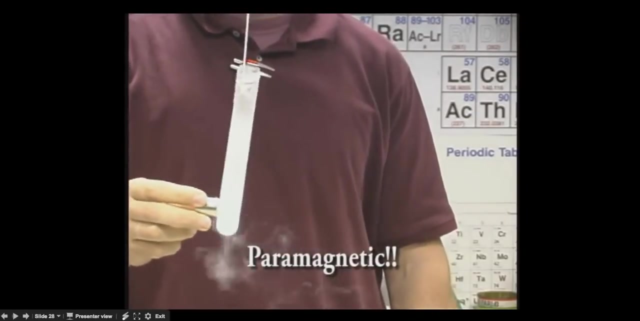 MO theory but not predicted by valence bond theory. okay, a magnet can interact with those two lone pairs in those anti-bonding orbitals. So here I come and you can see that there's paramagnetic ability. Okay, Really cool. 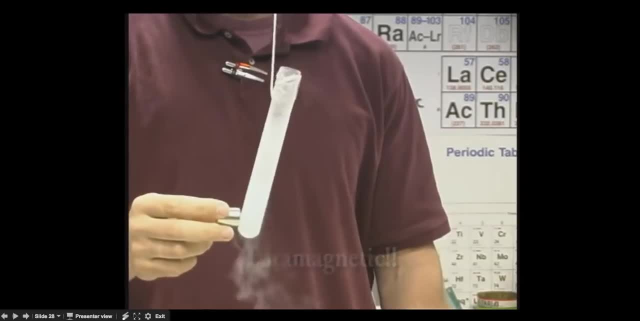 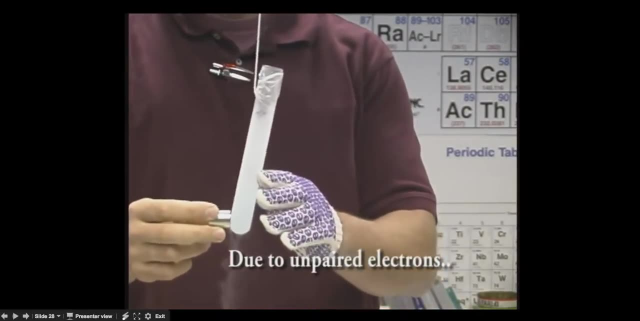 All right And no pun intended. Probably was a pun intended, So yeah. So essentially, again due to the unpaired electrons in the anti-bonding orbitals, again with valence bond theory we don't have that. 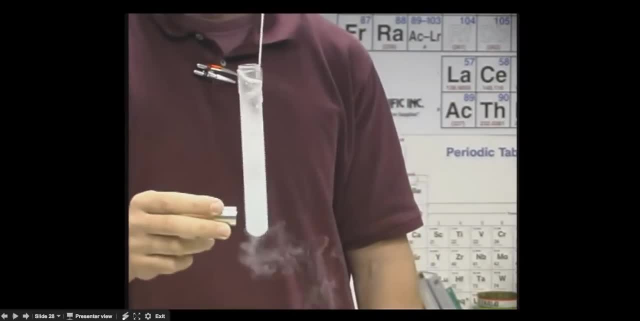 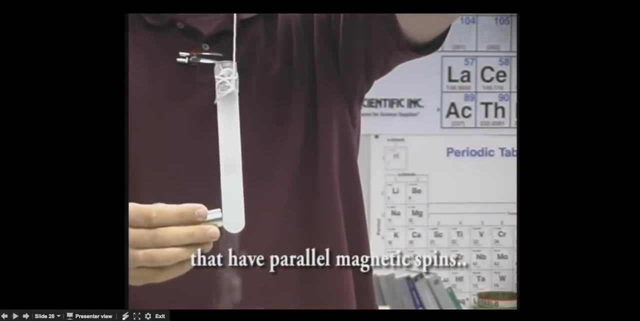 So that little gap from bonding to anti-bonding is enough to number one. have its blue color, but also give it its paramagnetic spins or its parallel magnetic spins, as I'm trying to read. All right, So I think you get the point. 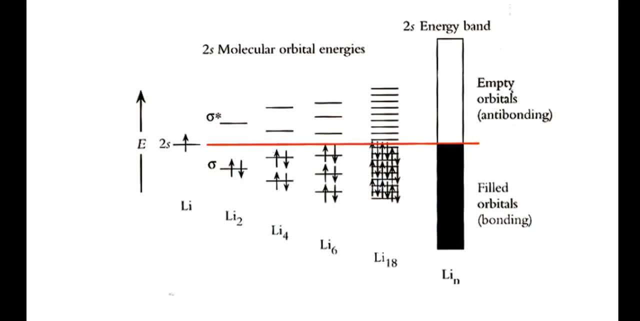 All right. So what we have here is a picture, maybe, of an MO diagram, Okay, And so we're looking at the. if you look carefully, we have lithium and then we have lithium-2.. So this would be the atomic orbital diagram. 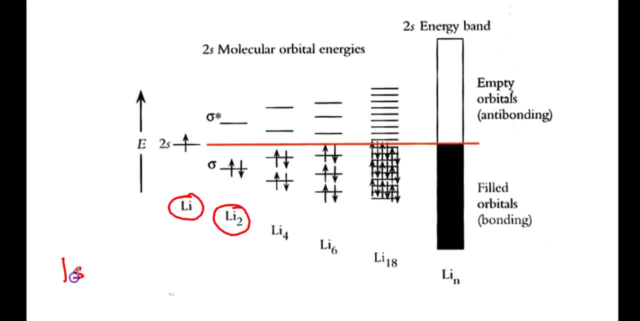 It has one electron. Remember, lithium is 1s2, 2s1.. We're just going to deal with the valence shell. Okay, Now this one electron is in the s Now when lithium bonds, as we saw two electrons go in the what? 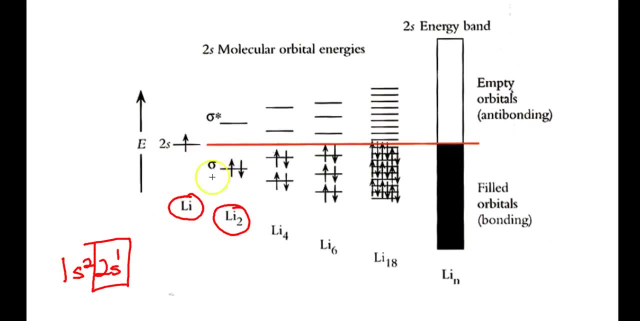 The sigma 2s orbital And it only has two. Now, if you add more atoms like L4, what you're going to do is you're going to add more orbitals. You see, you're going to add what? 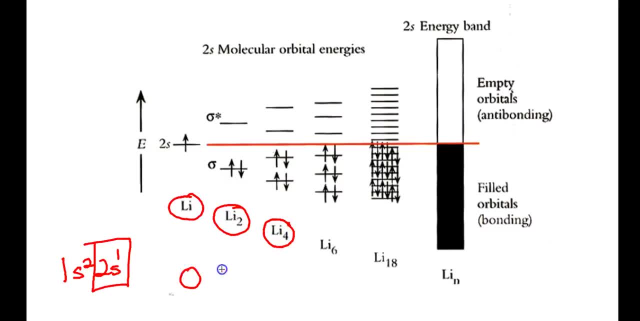 Well, four atoms, okay, are going to be 4s orbitals, So you're going to make four. well, actually you're going to make two sigma. So four atoms come together, okay, each with one electron right in the outer shell. 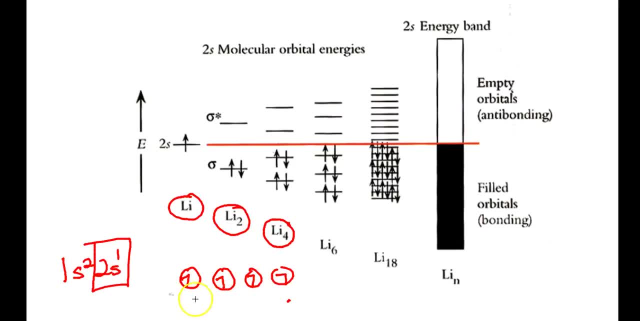 You put them together, you're going to make two new bonding orbitals, Okay, So what you're going to see is we keep putting our single electrons And what we do is, essentially, if we keep somehow interconnecting these electrons, we're. 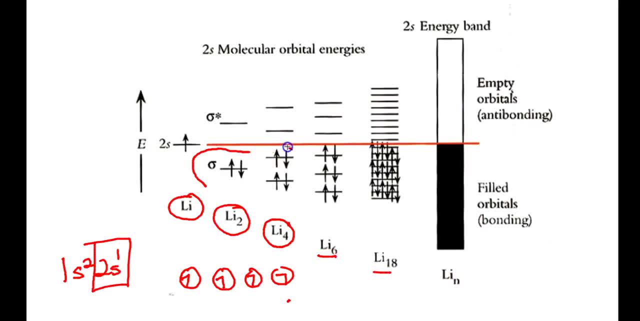 connecting these atoms, okay, we start getting what we call a continuum. So as we add more and more lithiums- now lithium's a metal and metals interconnect to make solids And as they interconnect, okay, where one lithium starts, another starts- we're kind. 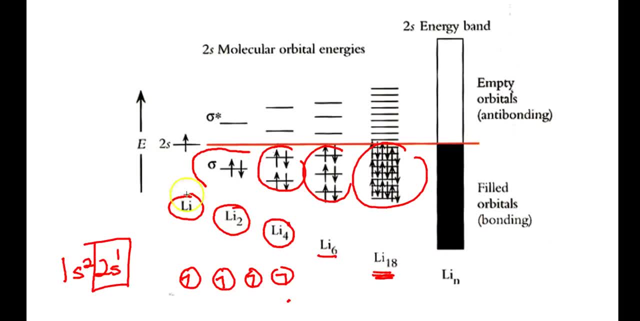 of making a super molecule. Now, they don't make molecules. we learned earlier on. There's this face-centered, cubic and body-centered type of arrangements, But the bottom line is we're creating bonds between the lithium atom. They're metallic bonds and you may have learned that there's a sea of mobile electrons when 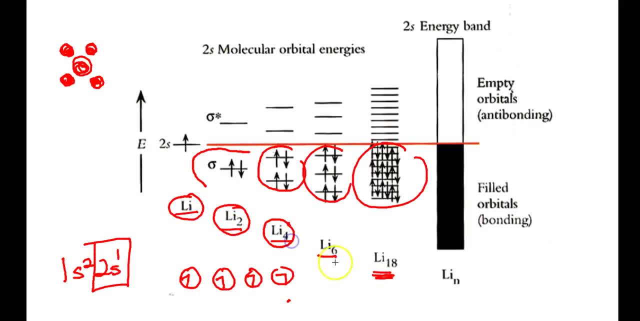 we have metallic bonding. So MO theory shows us that when I put these guys together together, I'm just putting more and more what Bonding orbitals together. And of course lithium-18's small. If I've got a gram of lithium that's stuck together in metallic bonding, I'm just putting. 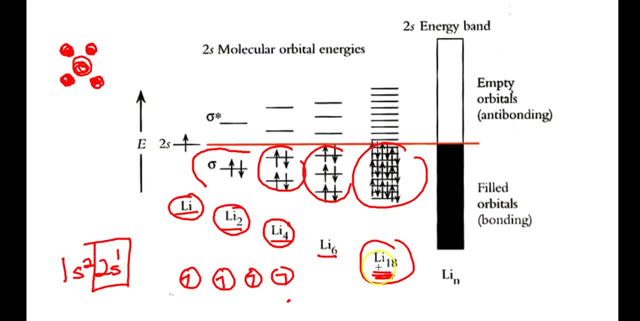 more and more what? There's a heck of a lot more than 18 of them. So these individual energy levels start blending together as you add more of them until, like I said before, you have this gap okay, or bonding gap okay, or this continuum. 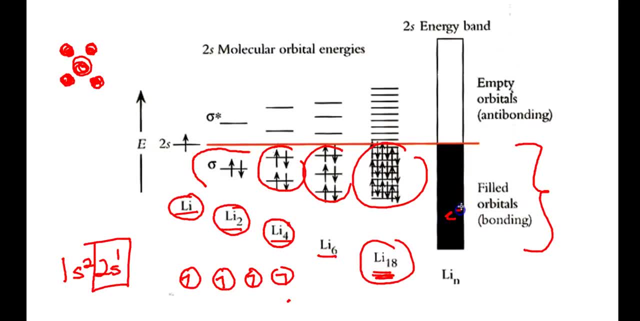 So this becomes electrons that are able to basically move through this entire region and act as a single energy level. Okay, So it's a continuum, So electrons don't have just this energy, They're basically able to move throughout all the orbitals. 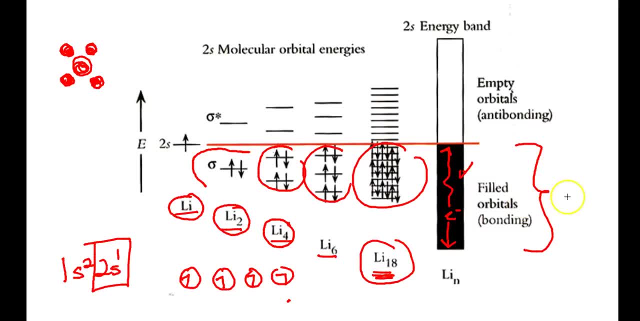 They're essentially at a single quantum level of energy that's described from this region here to, let's say, this lower energy. So there's a continuum. You can't say where one starts. They kind of all are inter-lapping. So basically, and if you remember in your earlier chem class maybe that metallic bonds- 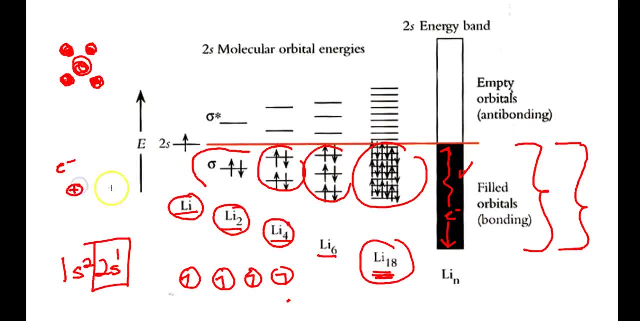 bonding, we have this sea of mobile electrons, If I have the nucleus- and electrons are able to move throughout the entire. what crystal structure of a metal we said that they're held so loosely? these electrons are free to move all the way around. 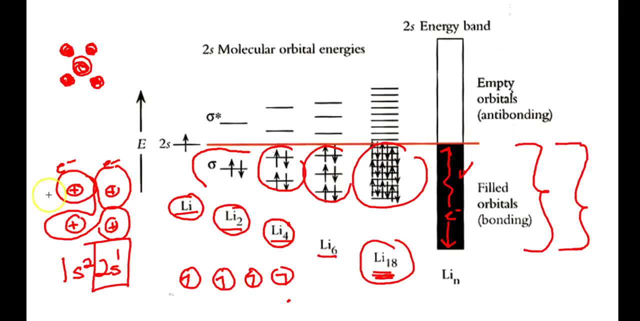 Okay, And when they move all the way around? that's the reason why they have conductivities: Electrons are loosely held and they're able to move throughout. Well, they don't really move throughout. They actually have this continuum of energy that they can move through here and higher. 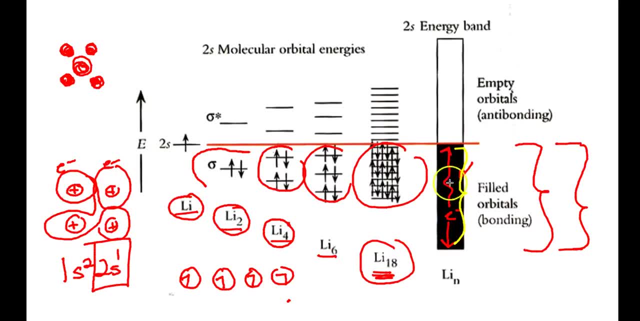 So they have a great swath of energy because they're able to kind of migrate through all of these orbitals that are blending into one. Okay. Now the anti-bonding region: okay, never gets any electrons in this scenario. okay. 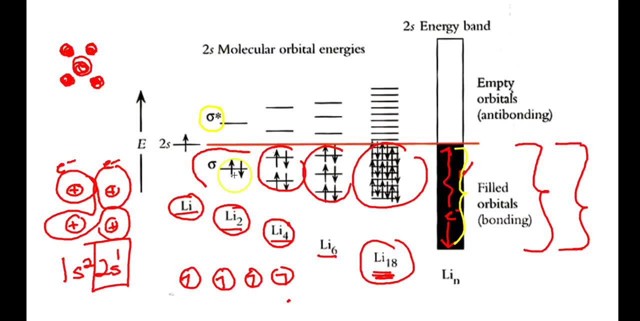 because we're always adding an electron to another region, Another bonding orbital. So we have room here. But what's really important is, the anti-bonding region also becomes a continuum as well, And we call this the conductive band. This is sometimes called the valence band. 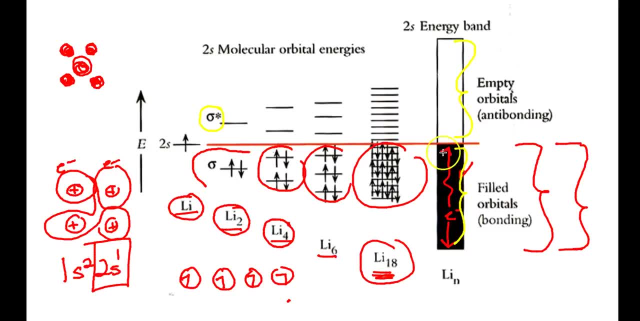 These are all the valence electrons and we call it a band because they're not in one energy level, They're in a gosh, basically a continuum of energy able to exist through all of these orbitals one the same. So it's kind of like all of these orbitals by putting together your MO diagrams are 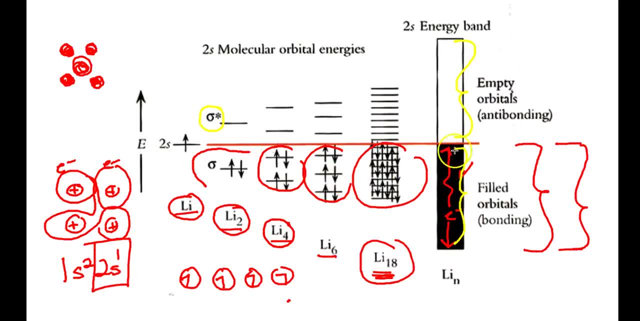 blending into just one big region of electrons that all have the same energy level. Okay, And if the anti-bonding do the same thing and we have a continuum like this, it doesn't take much energy, okay, for an electron that's in this gap to move. 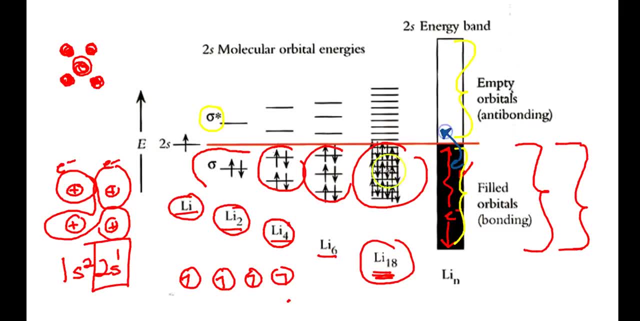 This gap, to get into this gap, this band- if you want to call it A continuum- is a band of orbitals- in this case, anti-bonding orbitals- that, again, as we increase the number of atoms that are interconnected, this gets smaller and smaller and smaller. 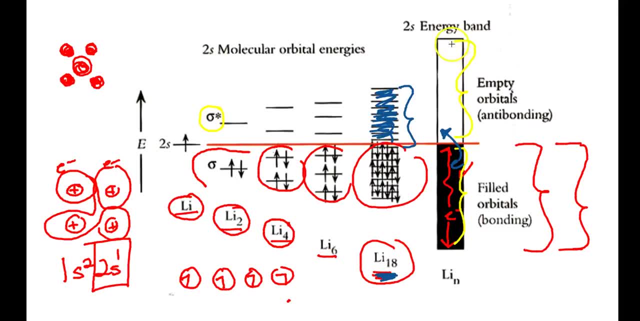 until, essentially, you've got electrons that can exist in this continuum, all right, acting as a single, all these electrons acting as if they have the same energy. But to get to this higher energy continuum or band, yes, you would need energy. 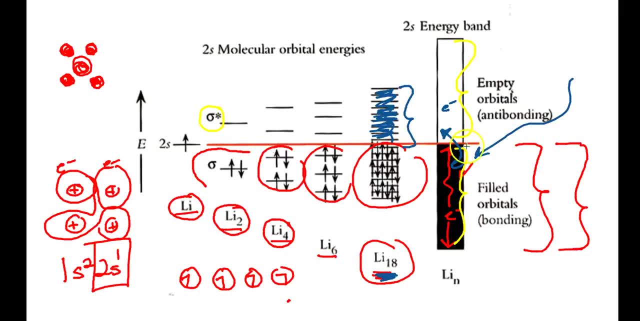 So things that conduct electricity very well have very small gaps between these continuums And again they're built because these MO diagrams are stacking on each other. okay, Very important. This happens all the time in metals, because in metals we say metallic bonding. okay. 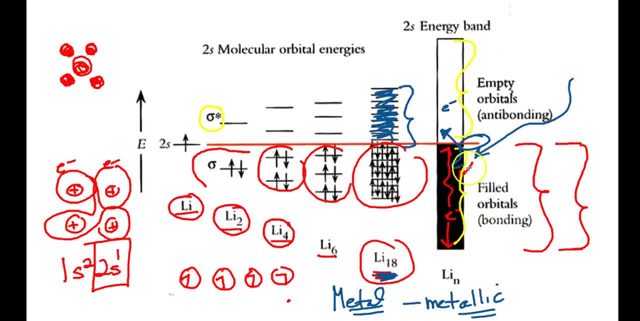 but really what it is is we're creating a continuum for electrons to exist throughout the entire molecule and, yes, they're able to flow very freely throughout this band, But, more importantly, okay, when they really really move, conductively speaking a little. 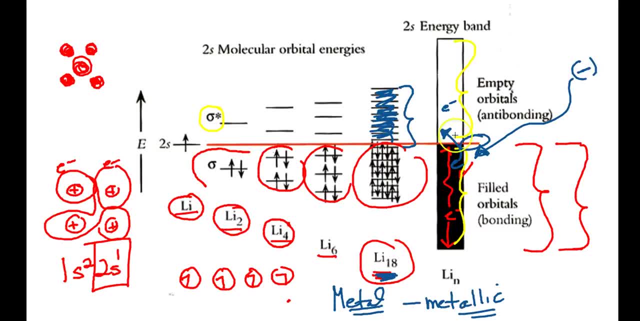 bit of energy is inputted like a charge or electron volt and they can pop up into this band here And I'll explain that next. Okay, So what you can do from this slide is that if you can stack these atomic orbitals, these 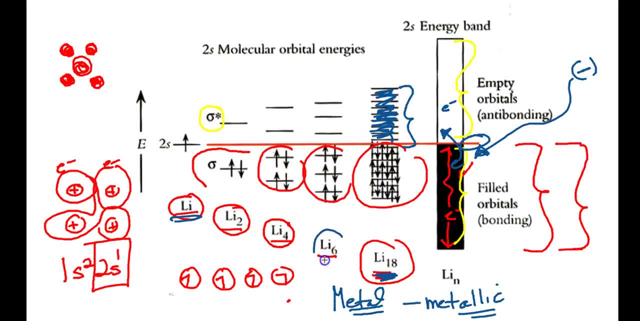 bonding orbitals and anti-bonding orbitals as you add more atoms together. okay, you create basically one energy level that all these electrons can exist at. Now, of course, it's a range of energy, but bottom line is all these electrons in this. 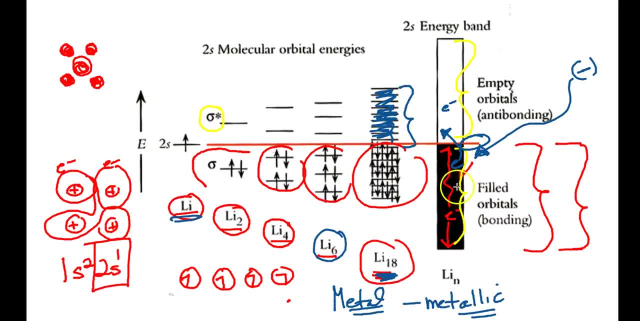 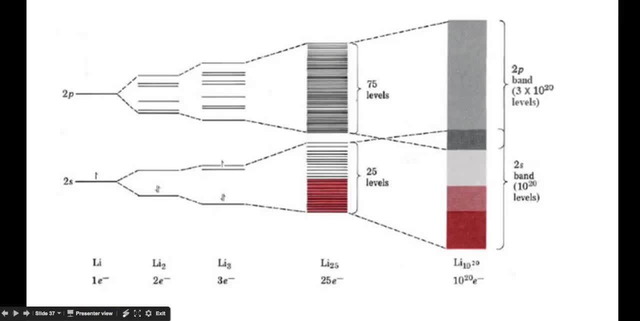 area, okay, are at the same quantum level. all right, So let's continue on. So here's another example. okay, Now this is the 2s bonding orbital and this could be the 2p bonding orbital, and you can see what we have here is we have overlapping continuums that occur, which means electrons. 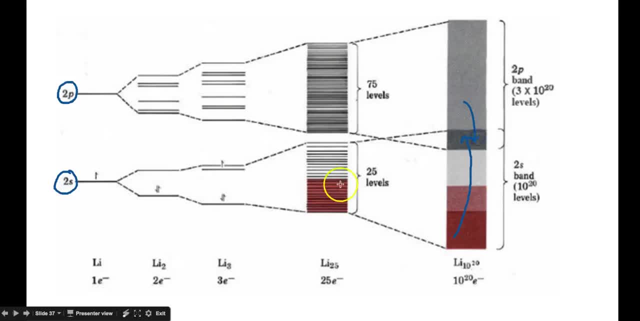 can freely get from one to the other, okay. Okay, There's an overlapping of these bands, and that's what you see with metals, is metals have overlapping of bands, meaning there's a way for these electrons to easily get to the higher energy position. 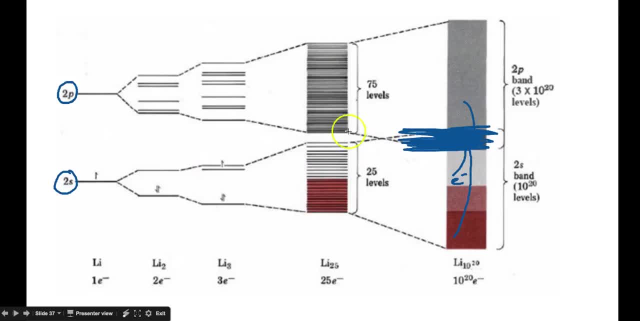 And if they can easily get there and get excited very easily with a very small- in this case no- gap, they overlap. these are great conductors because with a little bit of energy they can get to the next higher energy level. Okay, 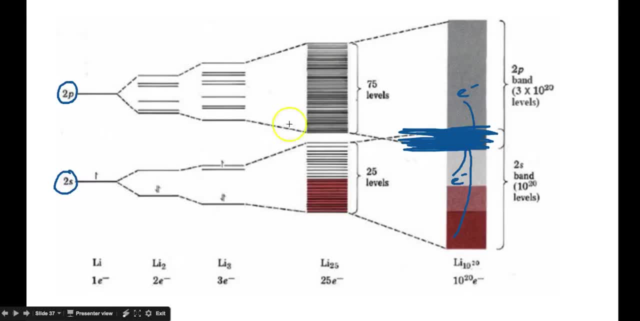 So this is going to be the anti-bonding, but this is the different type of p's that would overlap as well. okay, And look at the size of the 2s bands. okay, So that's what's happening here. 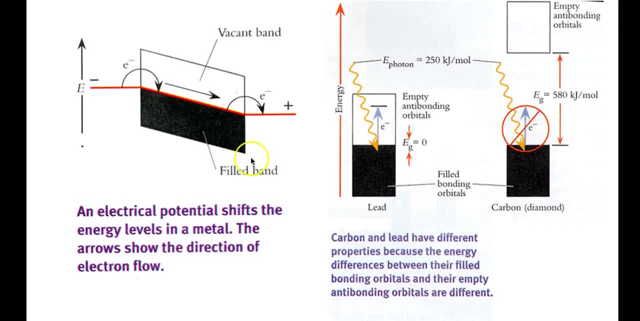 Let's continue on, All right, Moving forward. what we have here is we have this valence band- like to call it all right, And this is the conductive band. okay, This is the place where we have either an anti-bonding orbital or it could be another. 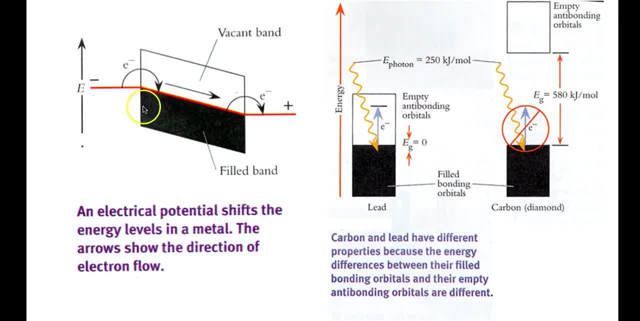 bonding orbital that it can jump to, all right. The bottom line is, with a little bit of energy electrons, can what Jump to the vacant band be excited When they jump back down they can give energy off to readmit one. 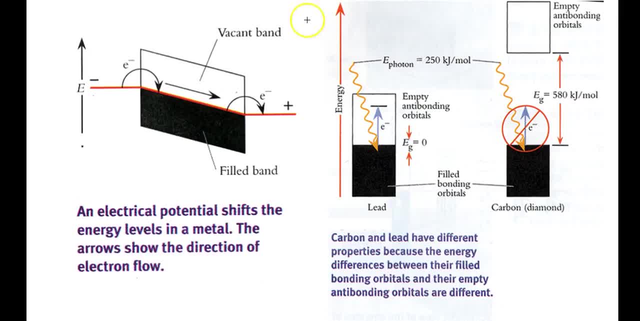 Let me just try to make some sense to that. So this really gives us a better view of how metals conduct electricity. So let me just make sure I get a nice little color here. So let's say I've got an electron here and with some energy I make a jump to the vacant. 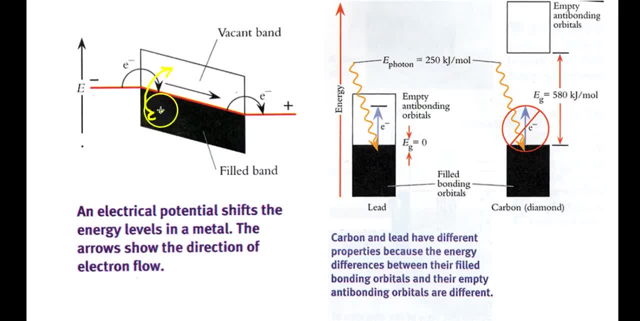 band. That's excited, Okay, And it won't take that much energy. Why? Because these gaps are really small. Sometimes they actually overlap, So this will jump down. When it jumps down, it releases what Energy for another electron in the vacant, in the filled band or the valence band to 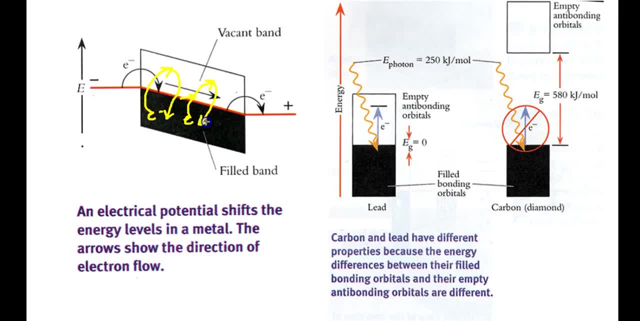 jump up, It's excited, It jumps back down, It releases energy for another electron to go up, and that's how charge is basically conducted. We're constantly getting exciting electrons with a little bit of energy. Okay, Electrons with a little bit of tiny energy don't need much. 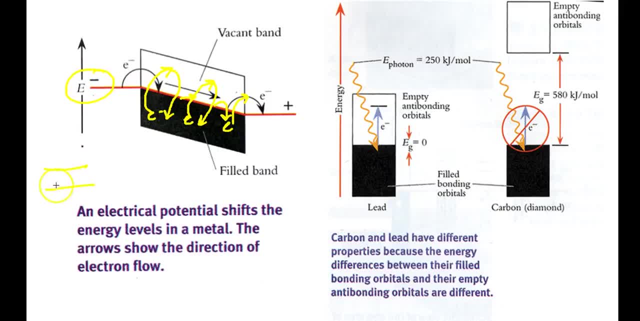 If what, The gaps are really small between the two bands or they overlap, Okay. So therefore it doesn't take much for the electrons to get to this higher energy position. They jump back, give off that little energy, and that can what? 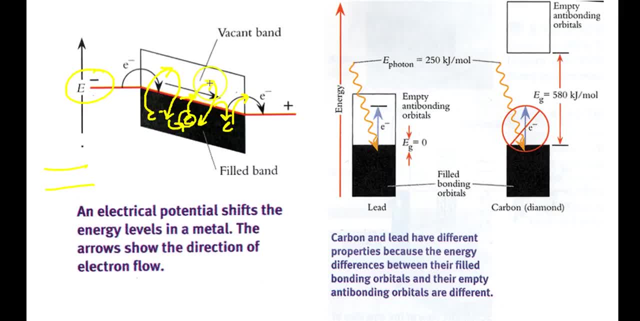 Re-excite the next electron who jumps up is excited, jumps back down, gives off energy, and that's how essentially electricity or electrical potential moves down through in all directions. Okay, We're pushing electrons into this vacant or higher energy level band, assuming the gaps. 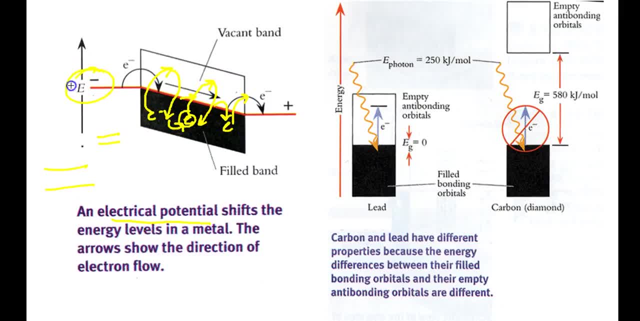 are small enough. If the gaps become too high and we too much energy to get this electron, you can guess what we have now is an insulator really important. So we look at two metals: lead in this case, and non-metal diamond. 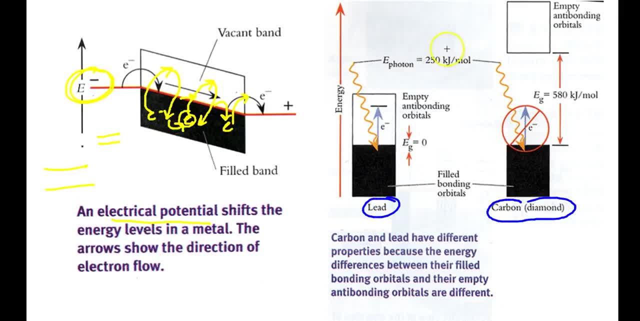 We know metals. okay, doesn't take much energy, let's say, to move an electron from the filled band or vacant band to the next band, because the gap is small, whereas the gap for a non-metal is much higher. hmm, very, very interesting. 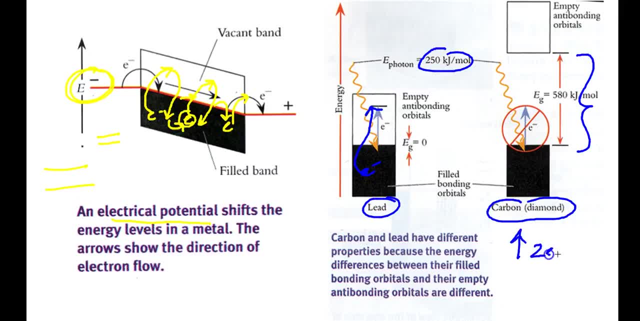 Carbon being a non-metal because it has a high ZEF. what does that do? Can't get away from it. It makes the gaps bigger. it pulls in these electrons in this band and therefore the gap between the bands, The continuums, are so big that it has difficult time for electrons to get here, and that's. 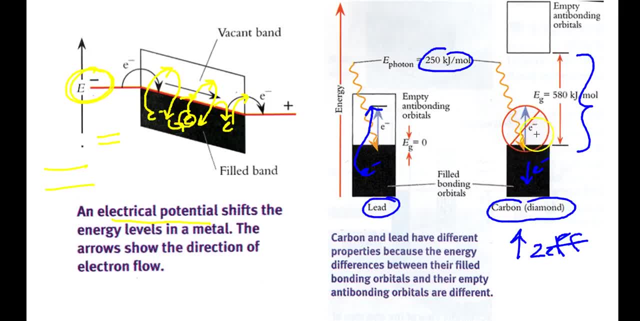 why carbon diamond is a terrible conductor of heat and electricity, whereas lead is much better. Okay, So the properties of our non-metals, our small atoms with high ZEFs are terrible conductors because that high attractive force electrons have contract these electrons closer to the 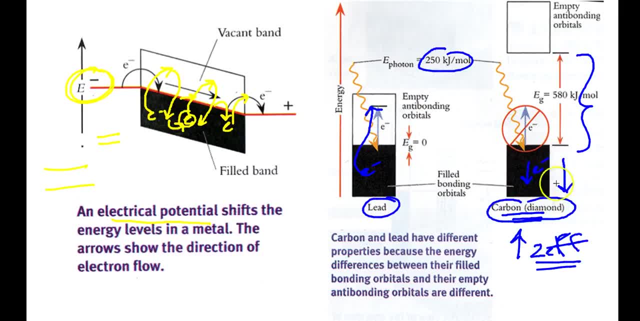 nucleus and make these bands smaller, Make these continuums so smaller That the gap from this continuum to the higher energy is too big. Sometimes they call this energy region the forbidden zone. okay, all right, and that's the area electrons can have. all right. 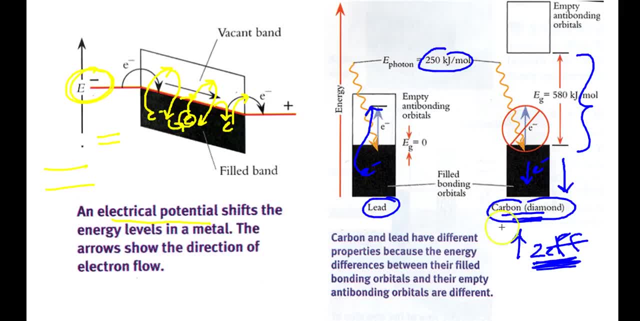 And it's all predicated about, you know, the structure of the composition of the substance and, of course, the effective nuclear charge electrons field. okay, Generally metals like lead have smaller gaps, Non-metals have bigger gaps, And that speaks to how hard it is for these electrons to get excited and therefore jump. 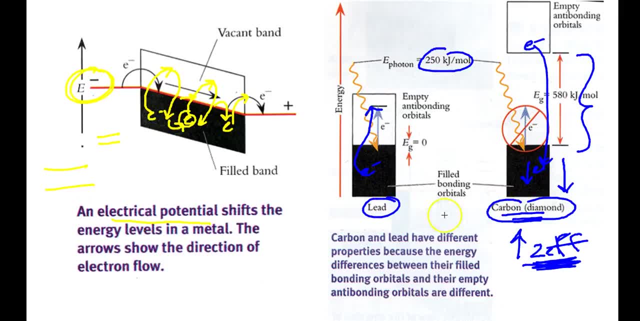 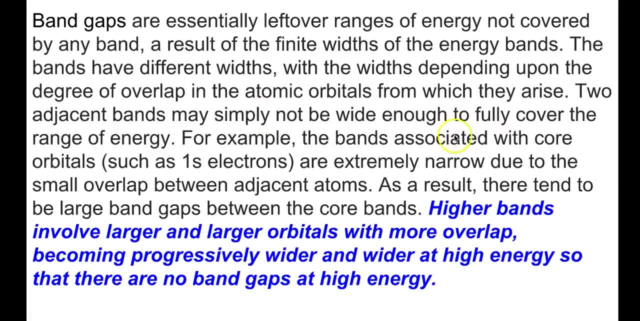 back down and re-excite another one, and therefore these are terrible conductors. where lead is better. Okay, Moving forward, Now you can read these. I have this same exact presentation on the site here, but really important point here, so I want to really kind of read it to you. 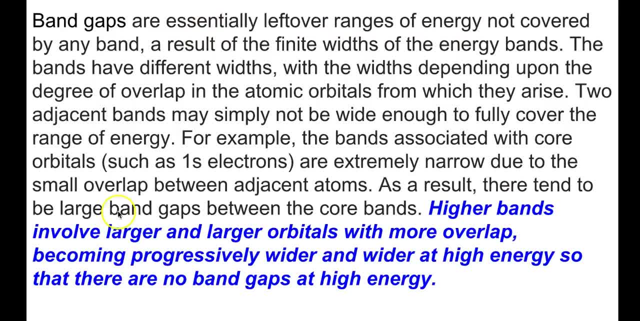 Band gaps are essentially left over ranges. So when you have a gap, okay In a Okay. So you have the filled valence band and then you have a gap for the vacant band or the conductive band. So here's our band, right here. 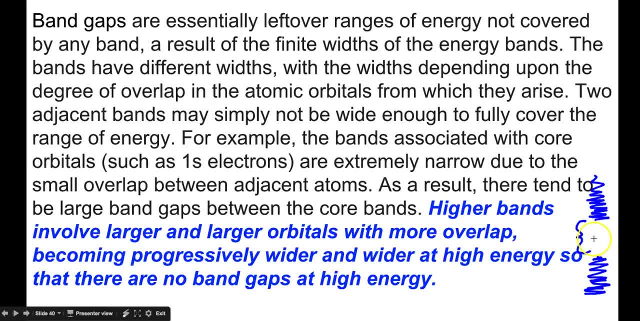 So these gaps or forbidden areas are basically left over ranges of energy not covered by any band, and it could be because we're dealing with very small orbitals. okay, and like the core, electrons are held tighter to the nucleus, they attract them more, so therefore they're 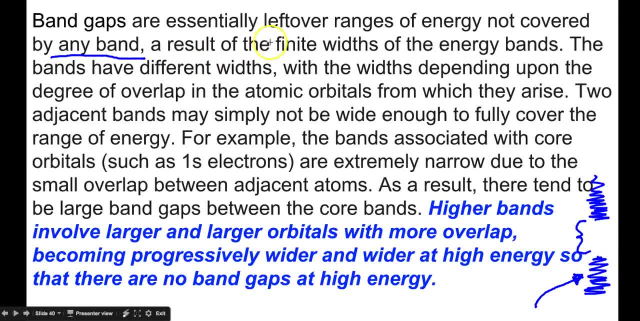 going to be smaller. Okay, So these are some of the reasons why, but the result of finite or definite widths of energy bands. So band gaps that we have are left over ranges that are not covered by another continuum. Okay, So the widths of these gaps depend upon degree of overlap of atomic orbitals. 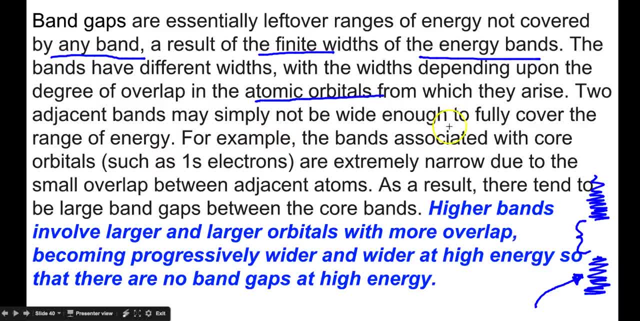 So very important. Two adjacent bands may not simply be wide enough to fully cover their range of energy, So this might be a 2p and this might be an s right here, Alright, For example. So the widths of these gaps that we're dealing with right now are extremely narrow, due to 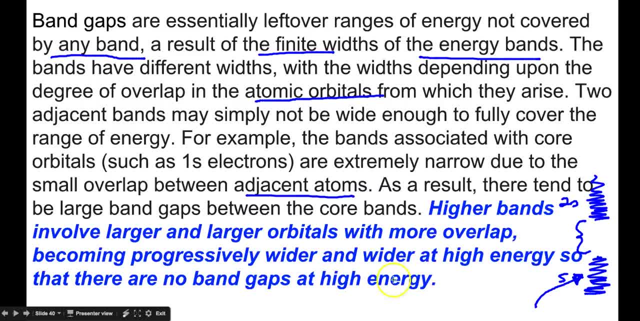 the small overlap between adjacent atoms. So we know that n equals 1, those are tiny, tiny orbitals, So their overlap is going to be so small compared to what Bigger orbitals, So therefore they have of course a smaller band and therefore that creates bigger gaps. 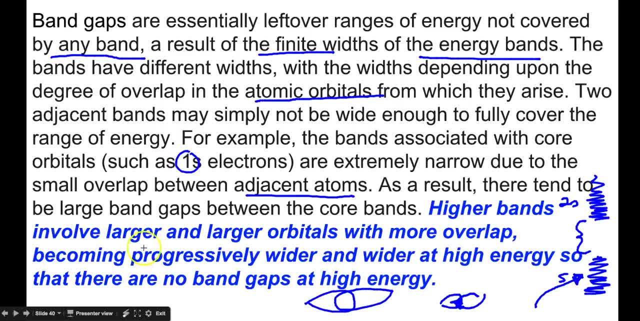 earlier on. Alright, So These atoms involve larger, larger orbitals with more diffuse electrons, more overlap. actually they're weaker covalent bonds and become progressively wider at higher energy. So there are no band gaps at higher energy kind of blend together. 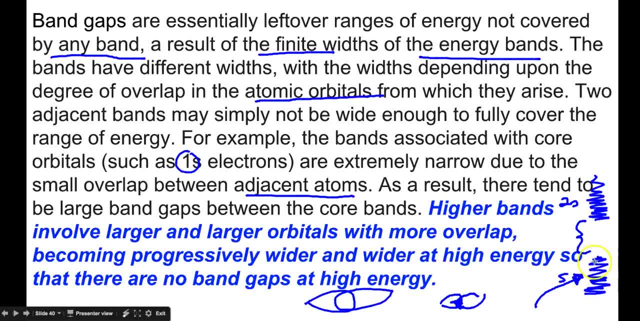 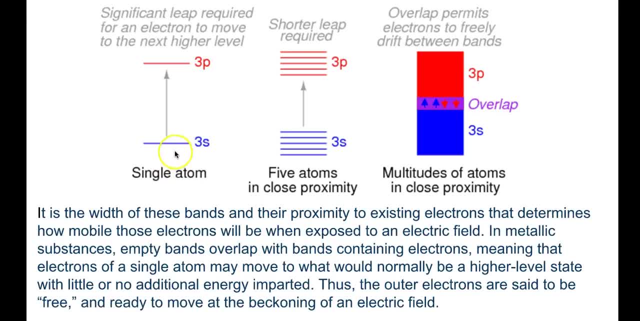 So the bigger the gap, the closer you are, the more electrons. and these orbitals are small enough, Okay. So, any case, moving forward. So when you have a single atom, you have atomic orbitals. there's definitely a finite amount. 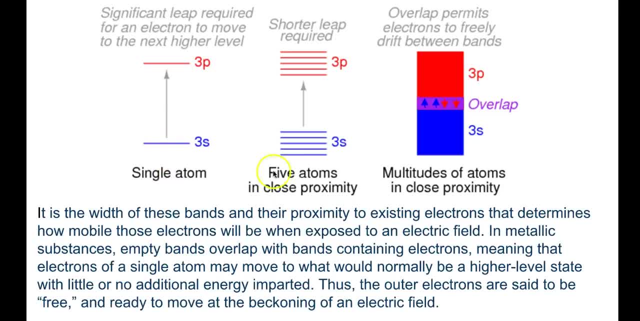 of energy to go from a 3s to a 3p. Now, When you have atoms, if their orbitals can interact- and there's definite ways they can- if they're solids, which means they're a continuous connection- of these things like lithium or 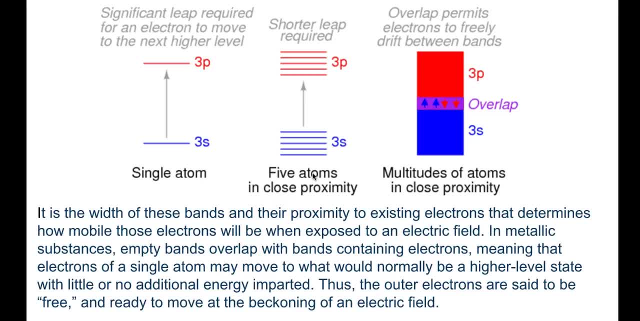 metals and even, you know, even like something like graphite, where carbon is bonded to carbon, non-metals bonded to non-metals. in that, in that arrangement, create these continuums as soon as like. of course, I've only have five. 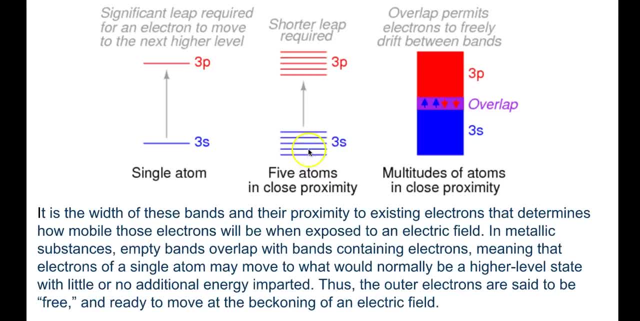 Okay, We start stacking these MO orbitals, Okay, And these electron gaps are really, really tiny, But eventually, when we have so many of these atoms that are interacting like a solid, okay, we can have this a continuum, and sometimes you have the overlap. 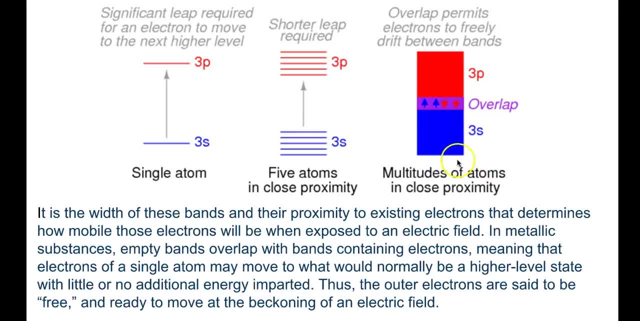 All right, Now they. once you have the continuum of all of these orbitals together, that will decide what kind of gap you have, based on the continuum of one to the other. Now here's 3s to the 3p, but it could be to the anti-bonding as well. 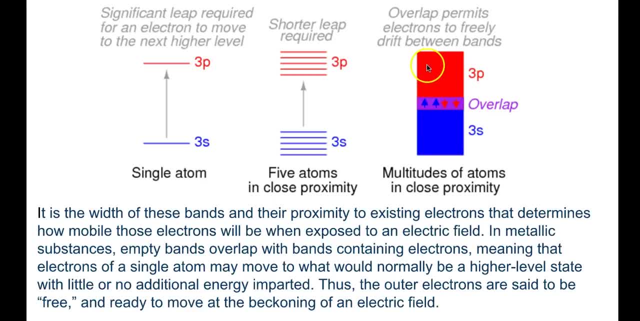 Like we talked about earlier, Oxygen's two electrons were in its anti-bonding, was able to jump. there was a little gap here, but that's not really gap theory because that was just basically two atoms- okay, interacting, All right. 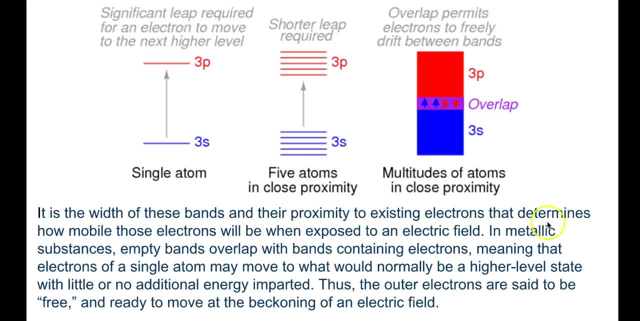 So it is the width of these bands and the proximity to existing electrons that determines how mobile these electrons when exposed to electrical field. So the idea is that these are mobile electrons that can occur in these bands and only occurs under a set of conditions, And those conditions are that they're kind of interconnected, so to speak. 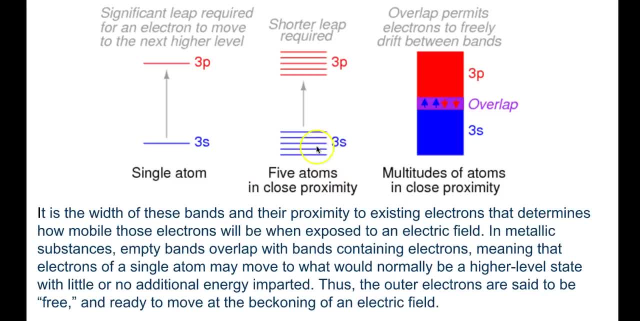 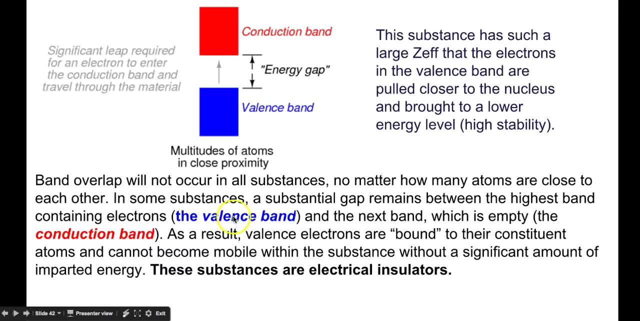 They can't be single atoms close to each other, like this is saying They have to be interconnected, So I'm not loving this. All right, Moving forward maybe. So here's our valence conductive band and there's a significant leap of energy into 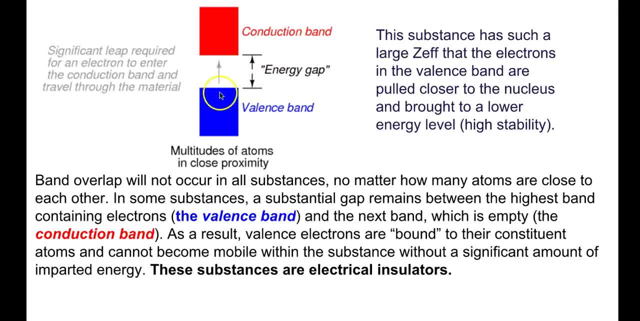 this energy gap or forbidden area. This represents something, if it's a big enough, like a non-metals, a non-metals and, of course, a large effective nuclear charge, It would do that And, of course, if there's a big enough gap and it's hard for electrons to move from this, 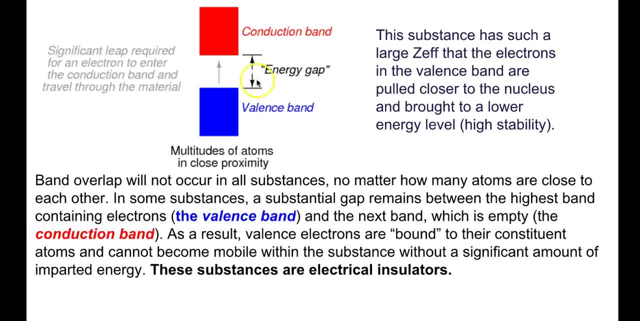 continuum to this continuum or this band to this band, a big enough gap. this would be an example of electrical insulators. So these are hard to get from one to the other and jump back. So as a result, we would see, electrons are more strongly bound. 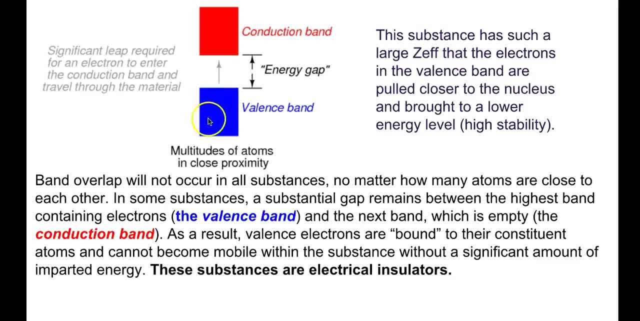 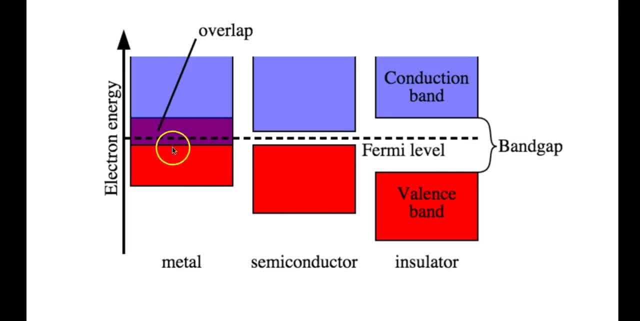 And of course this occurs with high effective nuclear charge atoms of the non-metals. So here's a great little diagram here Where we have metals where the gaps are overlapping. So it takes very little energy to get to the overlapping, if any. 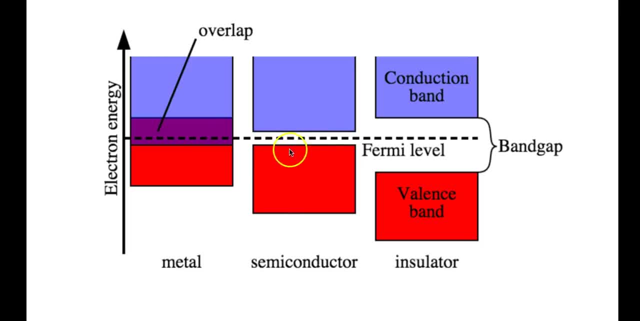 Semiconductors have a gap, which means they have a tough time getting there, but they have the ability. And then, of course, real non-metals, smaller atoms with high effective nuclear charge. their gaps are just too big. Their band gaps are too big. 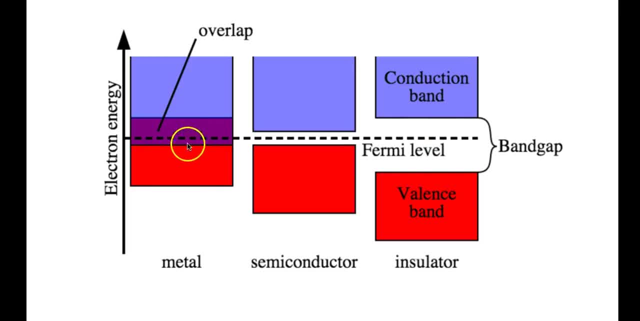 They're not good conductors, So metals have a very small gap, or just an overlapping gap. Semiconductor, as it says, it's not a great conductor, but it's somewhere in between that of the overlapping of metals and the big, huge gap. 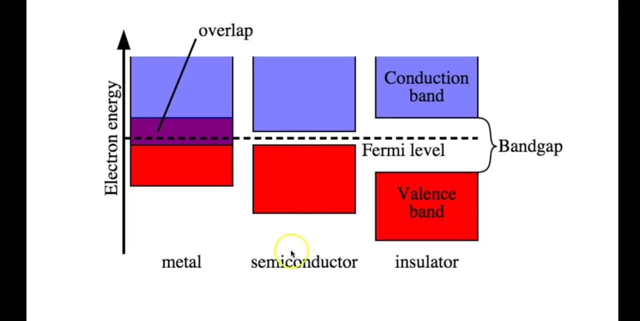 So they can have some conductivity And we're going to learn that if we dope a semiconductor, help it. we can actually change its conductivity by doping it, And we'll get to that in transistors. That's where we're headed. 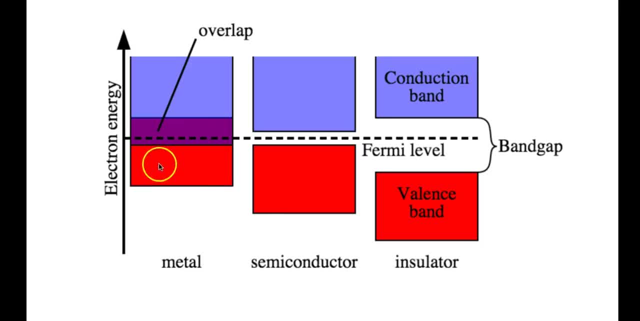 So MO theory And stacking the MO orbitals creates the bands depending upon the properties of the effective nuclear charge, or how these atoms can interconnect so they can stack their orbitals together depends upon the size of the gap. But the size of the gap drives the conductors from the semiconductors to the terrible conductors. 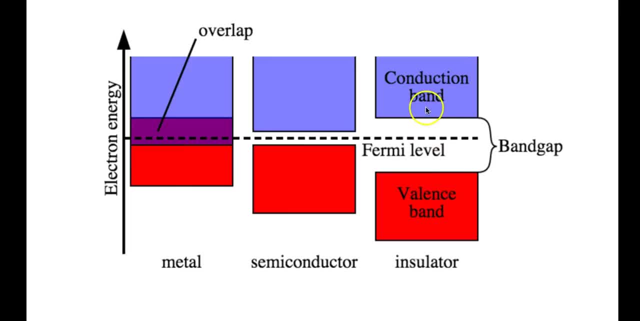 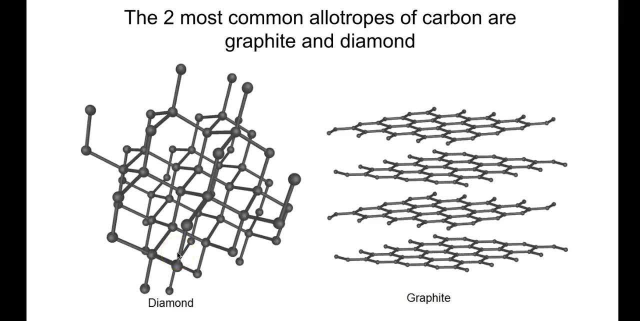 called insulators, So hard for these electrons to get to this level, So therefore they tend to insulate Heat And electricity. Okay, So we're going on to two common allotropes of carbon: are graphite and diamond? Okay. 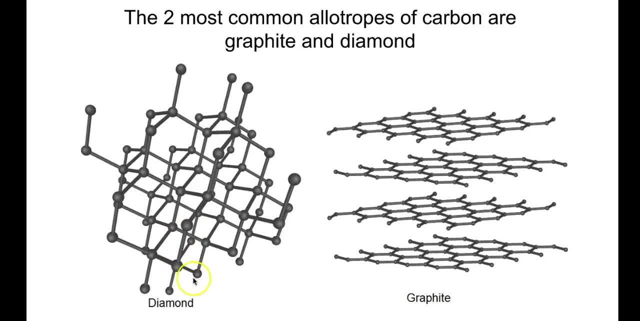 Now, diamond's hard to look at, but if you look at, carbon is bonded to other carbons in a crystal And if you notice it's bonded to four. So this is sp3.. If you look carefully, one, two, three, four- this is a tetrahedral that keeps going in. 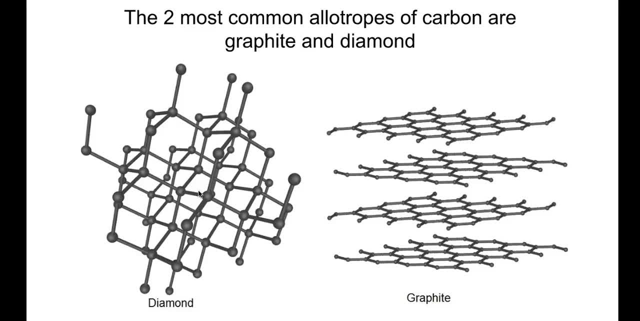 all directions. So this tetrahedral going in all directions creates, okay, this graphite, This gap or, I'm sorry, creates basically an interconnection of carbons with each other. So all the carbons bonding orbitals will band together to make a continuum. 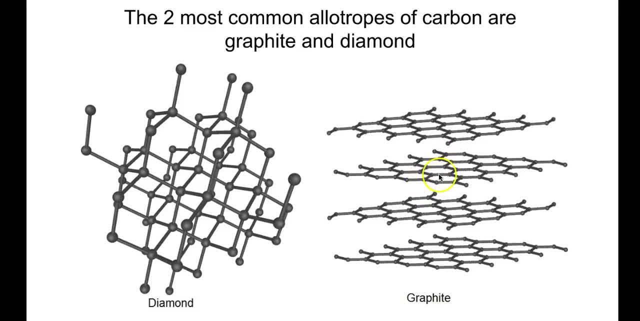 Just as graphite looks a little different, graphite, if you look very carefully, has essential carbon bonded to other carbons. Okay, So these compounds are rare in the sense that this is carbon bonded to carbon, what we call sp2, right? 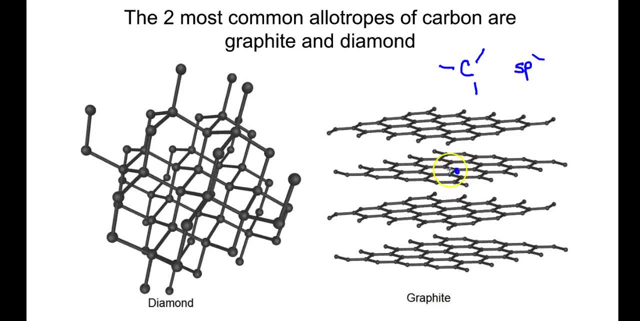 Because we have a carbon here bonded to three other carbons. You can count there. There's your trigonal planar. Here we have a carbon bonded to what? Four other carbons. So this is sp3, okay, But the bottom line is we're going to create bands or continuums, because these carbons 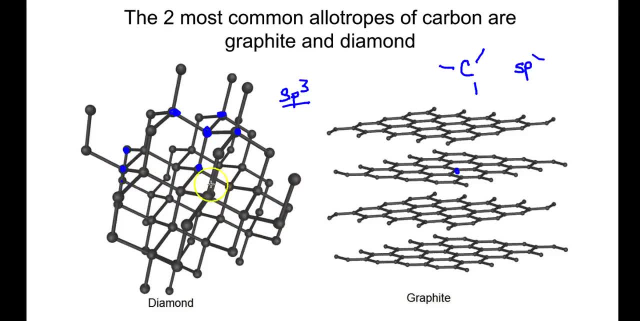 are totally interconnected, Every single one of these carbons, okay, Okay, They're sharing what or is adding to the MO diagrams. So therefore, we're creating bands. The question is, what kind of gaps are we going to have? As we talked about, diamond has a significant gap. 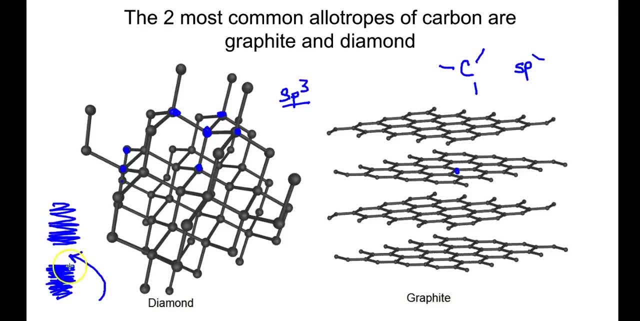 So, therefore, electrons have a tough time moving to this vacant band where graphite doesn't, And that's I want you to understand that graphite, now sp3,, these are all covalent bonds. By the way, it's called network solids, okay. 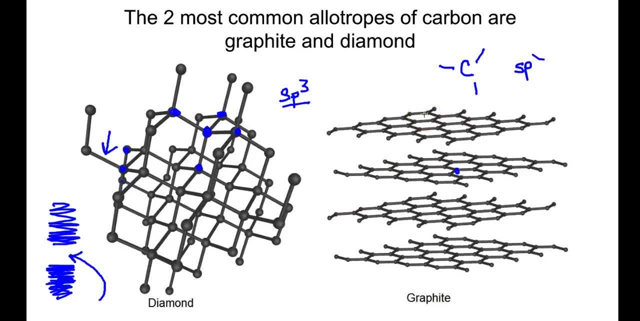 Because it's a network of covalent bonds. It's kind of weird because most things that are crystals, solids, are usually metals or ions, not things that are non-metal. But back to reality here. This is sp, I should say 2.. 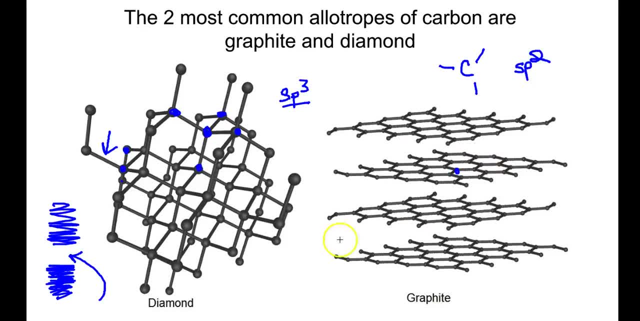 I'm not sure what happened there. This is sp2.. How do these sheets of carbon work? By the way, we have graphite in our pencils and they rub off layer by layer. Now, if it's sp2, what do we know? party people. 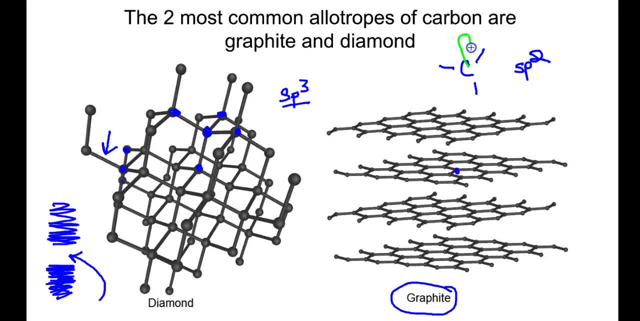 That there is an unhybridized what. This is sp2.. There's an unhybridized p. that's above and below. So every one of these carbons has an unhybridized p. So these have unhybridized p. 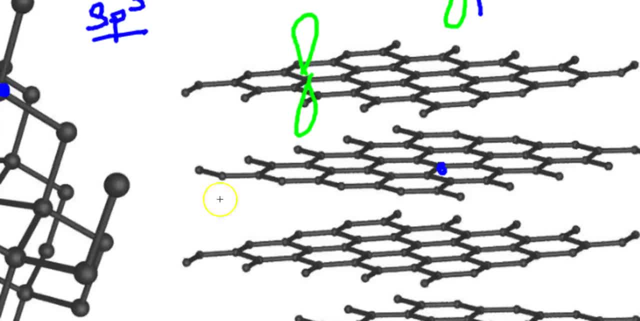 So really what you have? party people. I'm not sure why I'm zooming in, but I am okay. What you have is you have these p orbitals interacting with the other carbon's p orbitals. Now, I'm not going to say it's pi-bonding, but what we'll say is that there is an attractor. 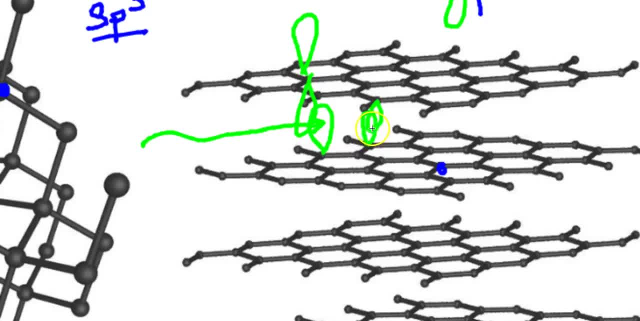 active forces existing. we think they're dipole-dipole interactions, but we're basically electrons are able to move throughout these p orbitals. okay, if everyone gives off a p orbital pointing downward right, these electrons can move throughout these p orbitals. 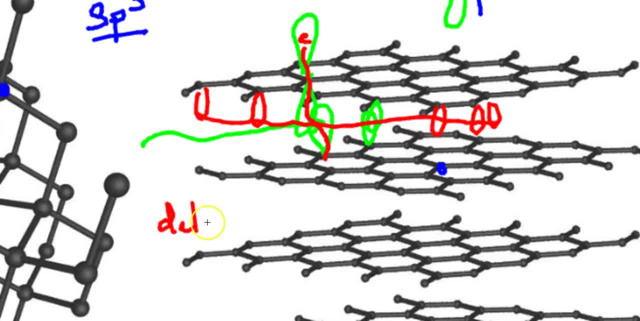 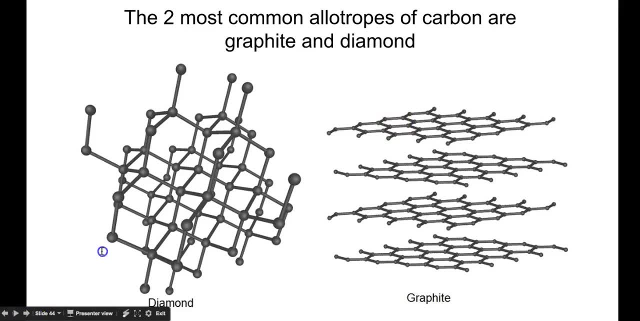 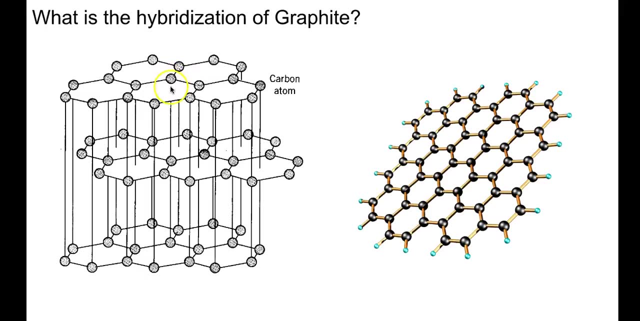 and be what we call delocalized. all right, And to see what I mean, let's go on to the next slide, maybe. So here's my carbon, here's my graphite, here's my sp. what two? and how does it interconnect? 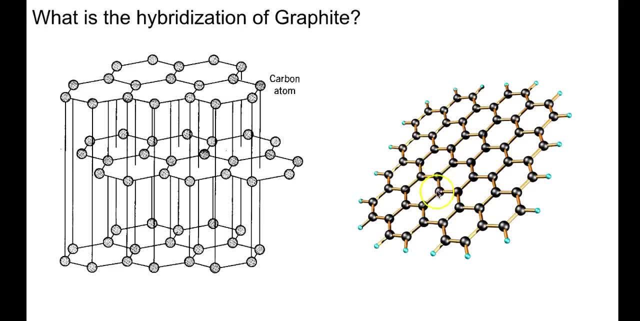 with the next sheet. You can see the sp2 trigonal planar right there. It's got these unhybridized p's that interconnect and make those electrons really delocalized. okay, So if we go on to the next one. so there it is. 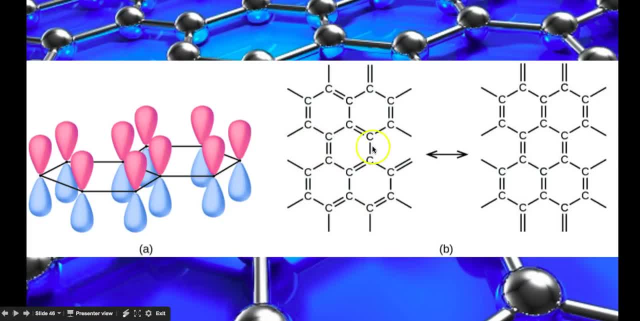 Take this trigonal planar carbons. and here's the planar carbons. Notice the hybridized p. So these electrons are free to what Migrate, which means these electrons are totally interconnected, and what we have is we have something called pi stacking. 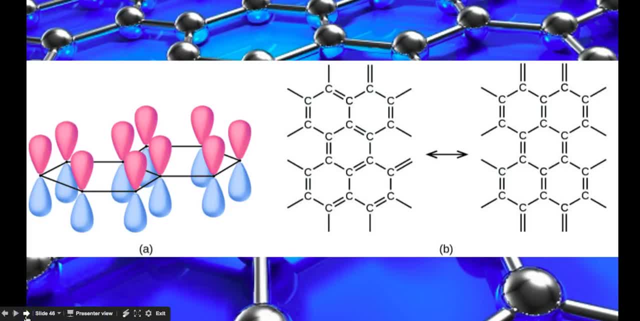 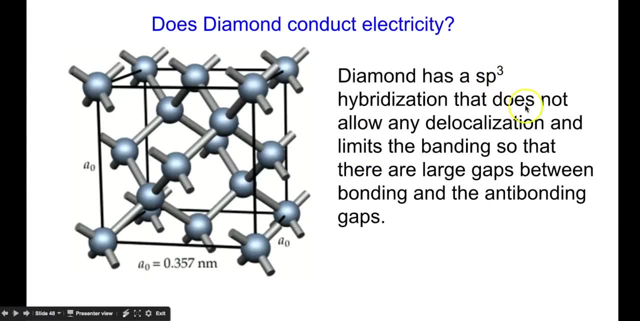 We're going to stack all these pi bonds in our mo orbitals. So diamond doesn't conduct electricity because the gaps are too big. The sp3 hybridization: The sp3 hybridization does not allow for any delocalization, So therefore it limits the banding. so there are no large gaps, okay. 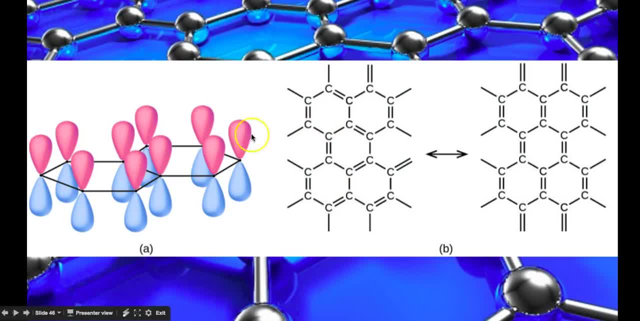 But what do we know? But in graphite sp2, with this unhybridized p where electrons are free to move around like resonance. and look at this: double, single, double, single, double, single. hmm, That's called a conjugation. 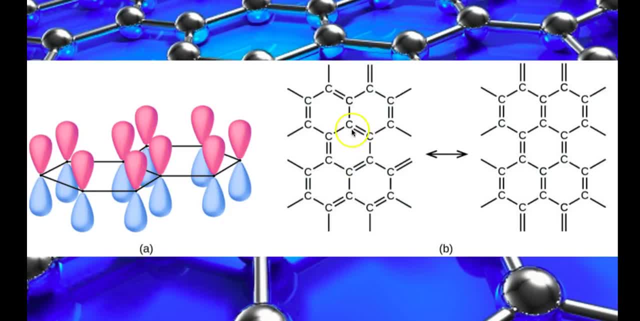 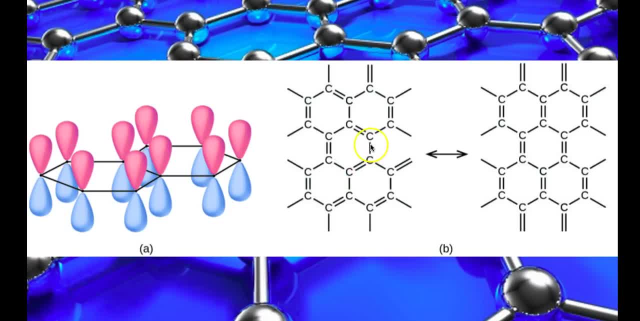 When you get a double single, double, single, double, single and this interconnects, all of these carbons must be sp2 hybridized And they all have an unhybridized p. So, unlike sp3 diamond, sp2 graphite has a way for electrons in the graphite to move. 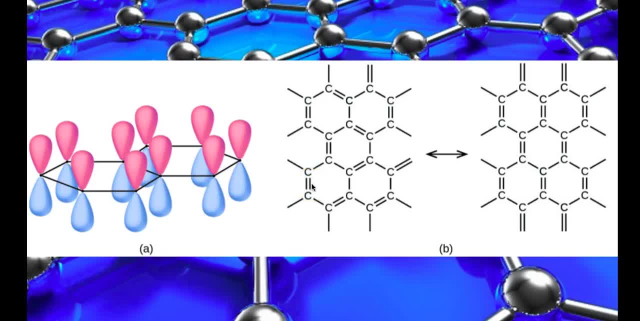 in these pi bonds. remember, every double bond is a pi bond. so really these pi bonds are resonating. There's a resonance structure. Look at this party people. It's going from this to this, back and forth. So really these electrons are able to move throughout the what? 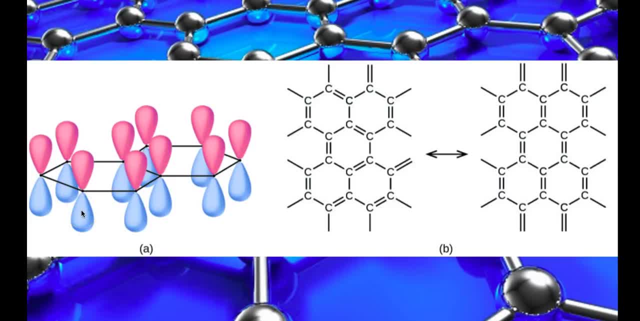 Unhybridized p orbitals, which means all the pi bonding orbitals are going to stack up nicely and make tremendous bands, Tremendous bands of very wide width. because there's so many of them, Electrons are free to roam. 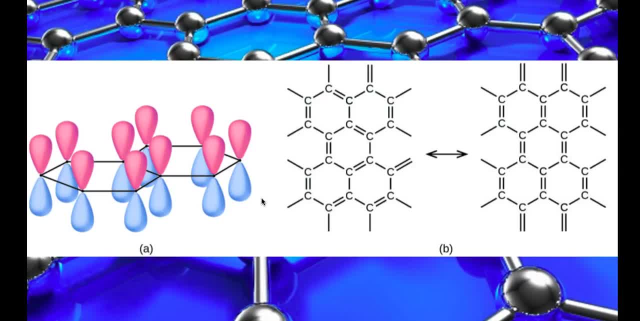 And, because of that, the gaps that we're going to make are going to be small enough for electrons to jump from a vacant band. And so, my friends in chemistry, we're going to be able to create tremendous bands because of what we call pi stacking. 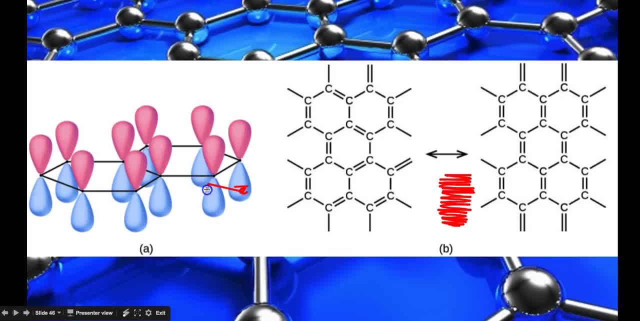 Pi stacking. So many of these electrons are free to roam, OK, and have delocalization, And we call this con- I can write here Maybe- And we call this conjugation: OK. Any time we have unhybridized p's and again we always have with a double, single double. 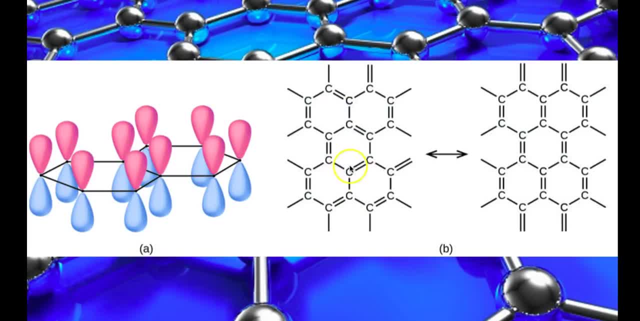 single conjugation that sp2 carbon results and allows for electrons to be delocalized. It allows for non-hybridized p's to be delocalized And that's actually a shape for all of these pi bonds to be part of the same mo diagram and therefore you're. 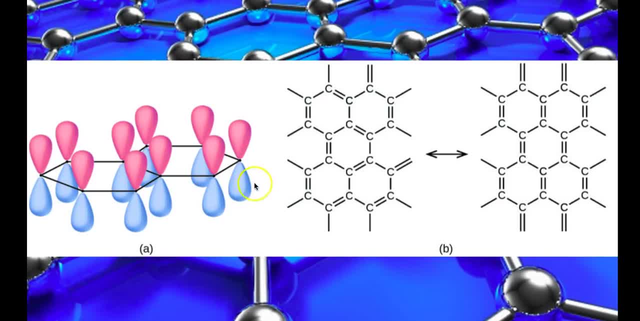 going to stack all of these orbitals into a major continuum, and there's so many of them, that is a great chance that band is going to be so small and therefore graphite conducts electricity okay, whereas, okay, diamond doesn't all right, very important. so if you're in, 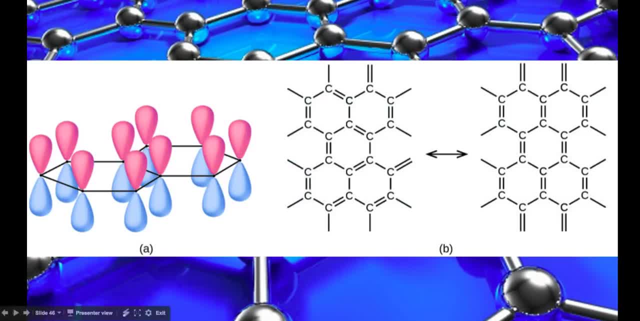 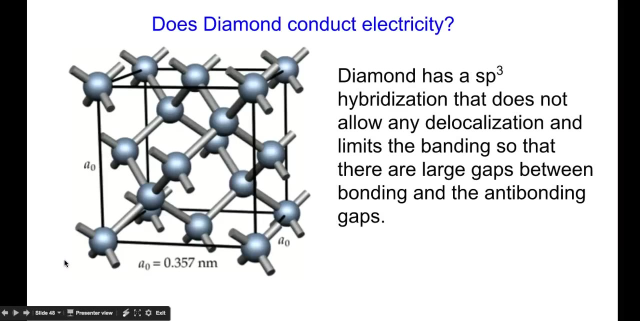 electrical storm. take it, take your pencils away, that's right. all right. so moving forward here, party people. okay, this conjugation opens up something called chromophores, maybe. so let's get out of this. and diamond doesn't conduct for reasons we just talked about, and now let's look at something called chromophore. 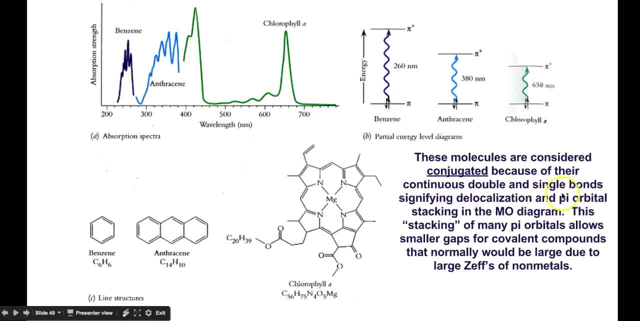 so these are conjugated because of their continuous double and single bonds. well, what does that really mean? double and single bonds means we have some type of energy that's going to be connected to a single bond and that's going to be connected to a single bond and that's going to be connected to a single bond. 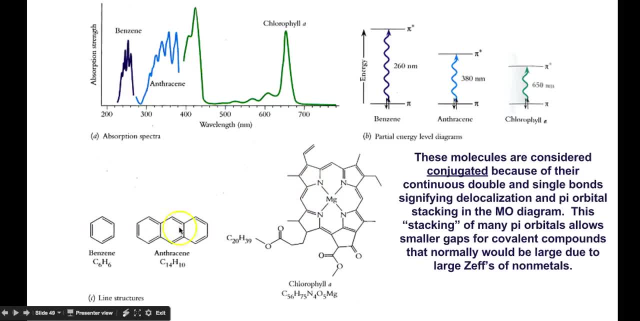 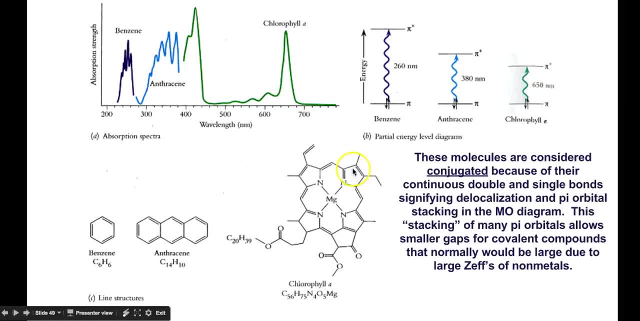 conjugated, double and single. you have unhybridized peas that allow electrons to be delocalized, which means you have a lot of what pie stacking, or a lot of the same pie bonding being the same molecular orbital, and that makes the gap smaller. so if we look at something like benzene, okay, if 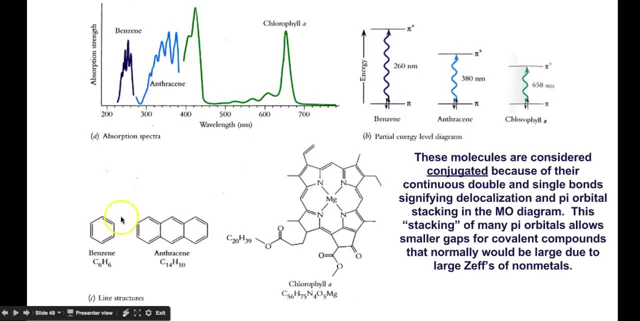 you look at the double, single, double, single, double, single. benzene is hybrid. I'm sorry, benzene has resonance and it has these sp2. nice, I'm mr Gretzky. I don't see the three. there's gonna be an electron that comes off this and these. 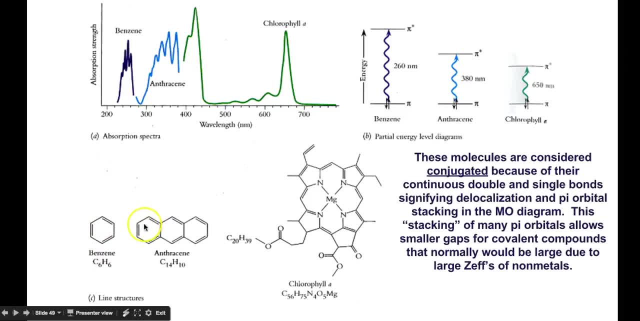 type of diagrams. they don't show the, the hydrogen. so with a hydrogen compounding coming off this corner- and this corner is a carbon, these corners roll sp2, which means they all have unhybridized peas, allow electrons to go in a circle. okay, and that's why sometimes they'll write benzene this way. okay, they'll write the. 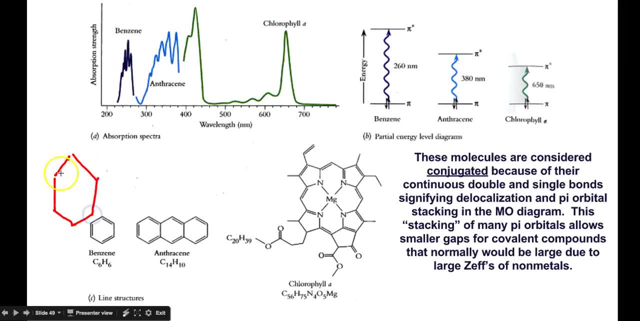 this, this, this, and sometimes remember I can put a double bond here, double bond here, remember, the corners are the carbons. right, okay, this is not a pretty drawing, but neither am I, and of course you can put a double bond here. and that's how the insulating Advil ratio thing is going to. 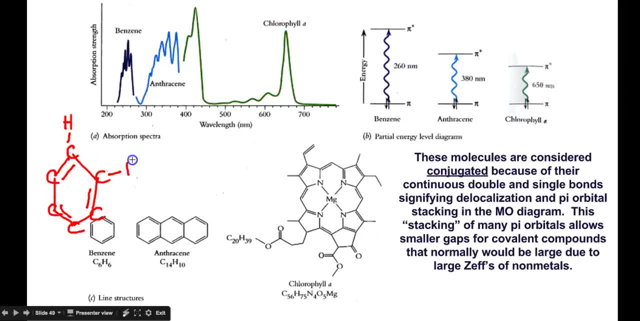 run. if they don't have a double bond, it'll be worth it anyway. the Тутwier one love award goes to this one here. this one here, this one here, you know, gives us one bond each to provide a new during. so you can, you know, humanity. 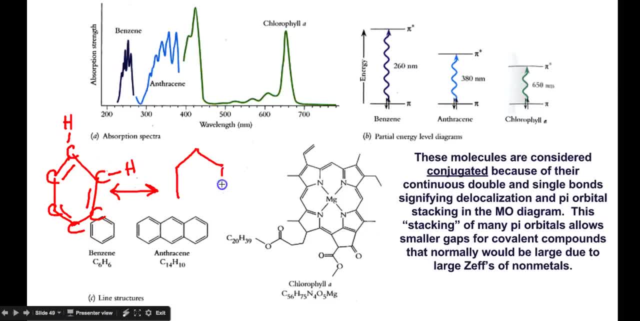 here is it go ST kidding. increases and increases, that's it all right, and- and actually I'm gonna- this is a pretty fun thing, globular even. but what are we gonna do, excited about it? Now, some people write benzene like this and they put a ring in the middle to show that those electrons from double to single to double conjugated, okay, allow electrons to just kind of continuously move. 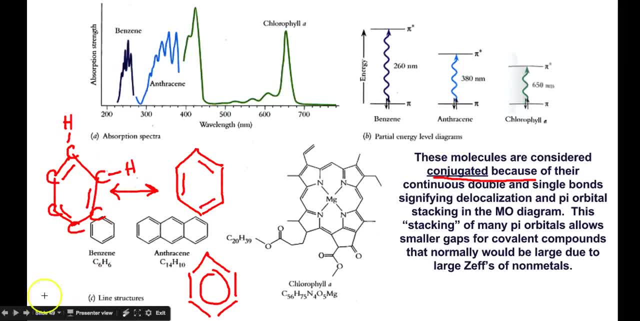 So benzene has some conjugation, Therefore it's going to have some continuum of those pi's, But those gaps are going to be pretty big And so benzene, if you look up here, absorbs spectra in the 200 to 300, I don't know about 250- range. okay, 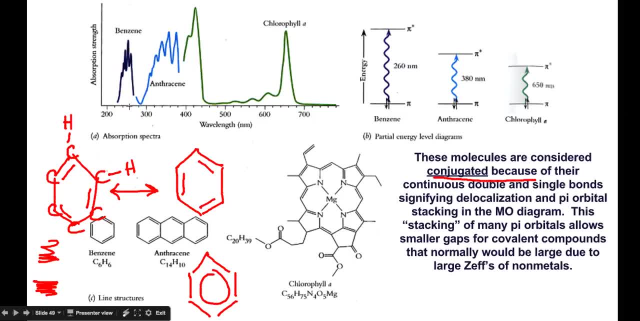 So that's not really in the visible spectrum. That is a pretty. this is wavelength, so the wavelength is too small. so it's really, really, really beyond the visible spectrum. So you would say that this is probably in the ultraviolet spectrum. 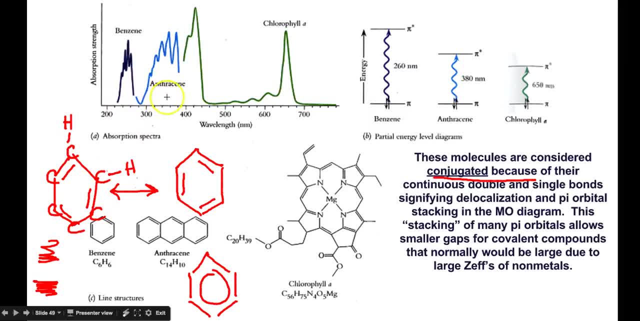 It absorbs energy. so that's why benzene is going to be clear. Now anthracene, you'll notice it has more conjugation. Again, look at these corners. These are all sp2 carbons, so they have the ability for electrons to travel through all of their unhybridized p. 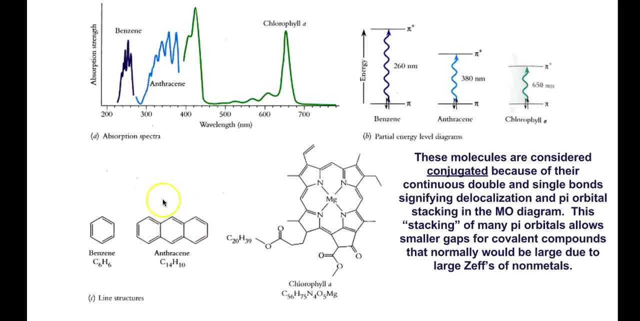 There's more conjugation, so there's more pi stacking, There's more orbitals, just like we did lithium, lithium-2,, lithium-3, and you saw the gaps become small and small until it was a continuum. These are making more of a continuum and the gaps are kind of what smaller, so now the wavelength it can absorb is bigger. 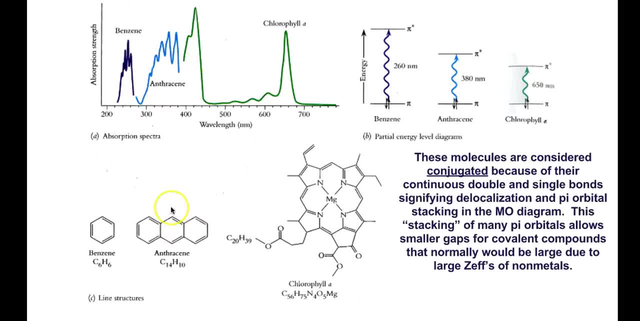 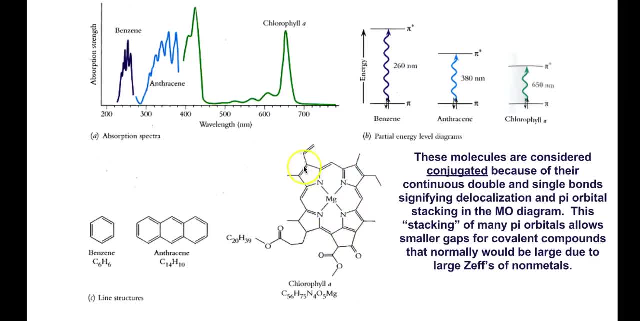 Okay, 1,, 2,, 3,, 4,, 5,, 6,, 7,, 8,, 9,, 10, I can keep going. Look how many places the pi Bonds okay can interconnect. so there's a lot more pi stacking here. so therefore, chlorophyll A: okay, can absorb. okay, in an even smaller energy level: okay, in the red part of the spectrum, okay. and also- I'm sorry, this is the blue part of the spectrum and this is the red part of the spectrum. 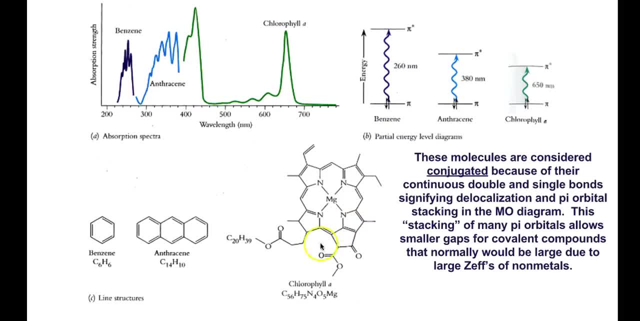 It doesn't do well in the middle, but and that's because of its complicated shape, because it has some conjugation that's kind of tied off and some that can go around in a circle. But the bottom line is it's more in the visible spectrum, it's more with the wavelengths that have what longer wavelengths, lower energy. therefore the gaps are what smaller. 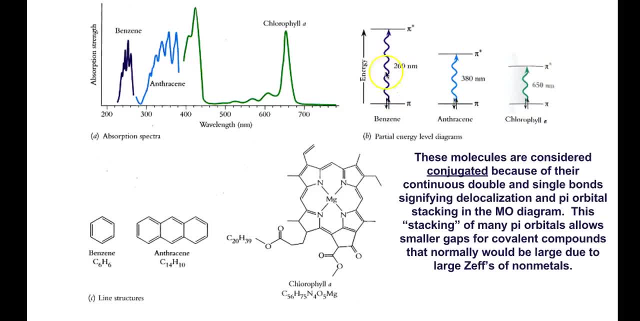 So benzene can absorb only big energy photons like ultraviolet. because the gaps are too big, because there isn't a lot of connected orbitals, But as a number of connected orbitals and unhybridized pi's and more delocalization, because of this conjugation the gaps get increasingly smaller. 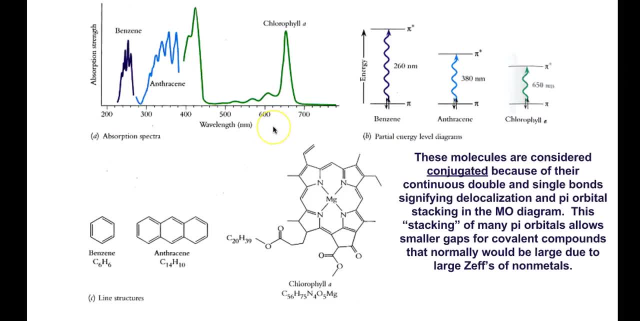 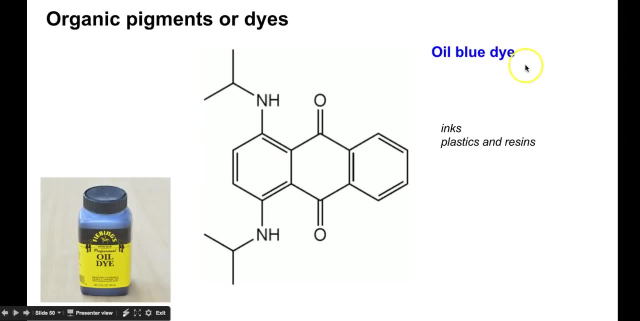 Okay, very important. So pigments or chemicals that we use that have color are able to absorb parts of the color because their gaps are smaller. okay, So if we look at organic pigments or dyes, this is an oil dye, which means it's blue because it absorbs the yellow part of the spectrum. 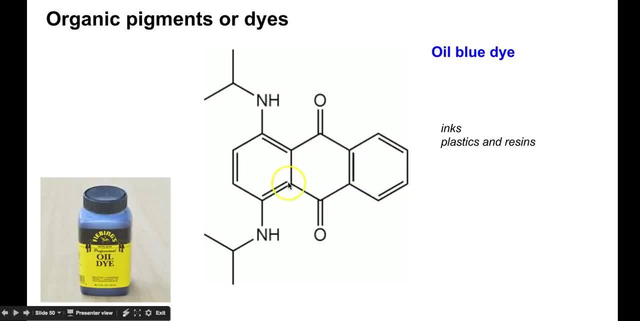 Can we see something? Can we see conjugation? Yes, you bet you can. These are all sp2 carbons, So the electrons are free to roam. okay, which means it absorbs the yellow part of the spectrum. It's got a very small gap. 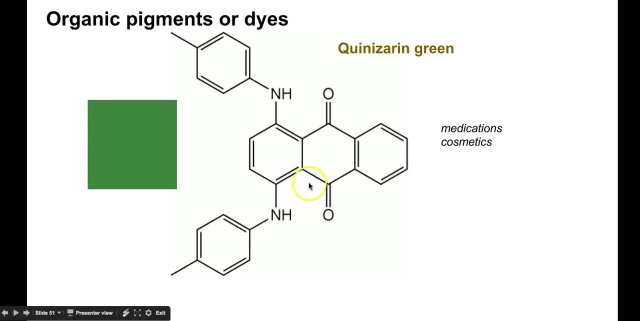 Now, if you look at other dyes- okay, here's green. Wow, that was yellow. Now this has even more conjugation, so the gaps are even smaller. But again, there's a little more complexity here with the N. 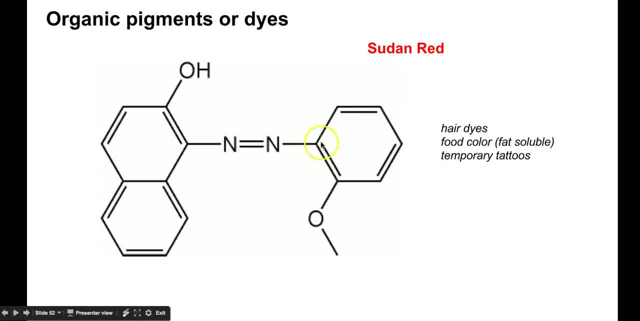 So what you're seeing with these organic dyes is the idea that electrons are free to move through these pi bonds. because of what? Because Because of conjugation or resonance. This delocalization of electrons allows all those MO orbitals to make a continuum. 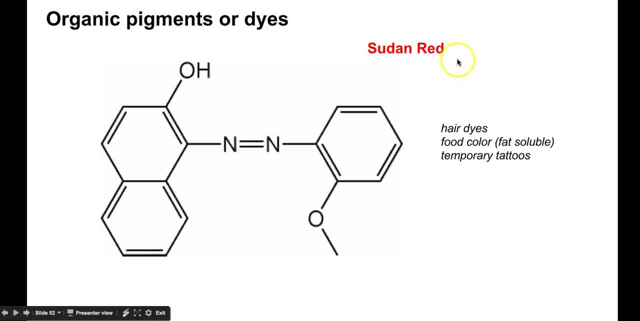 And the more you have, the smaller the gap and the ability to do. what Have a small gap from your valence band to your conductive band or vacant band. So all of these organic pigments that we know of all have something in common. 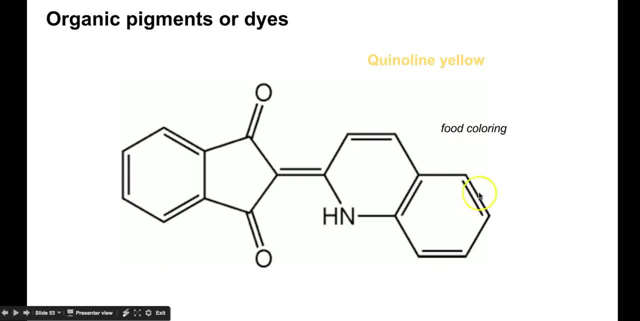 They have conjugation, We call these chromophores, We call these all dyes, And so we talked about earlier in the course, very interesting, about the transitional elements making colors. Well, these are how colors are made: with organic or nonmetals. 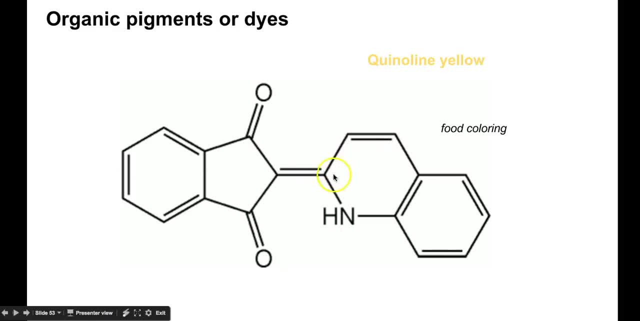 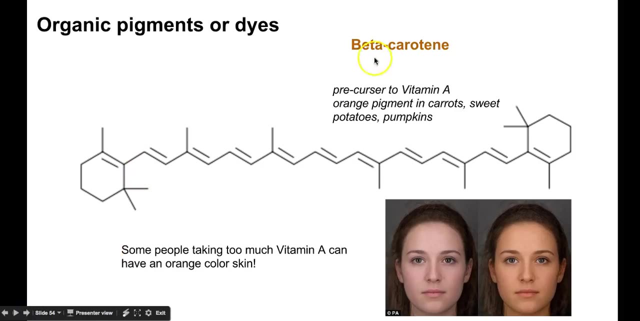 They have to have pi stacking in MO diagrams to create band gaps that are small enough. You have to have interconnected electrons sharing essentially The same energy level, So all of these dyes are connected by that. So this is beta carotene, SP2, all the way. 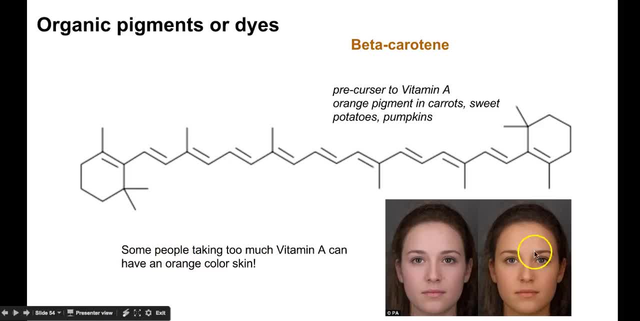 Obviously, if you take too much vitamin A and beta carotene, you glow an orange. So you can, because it's a fat soluble vitamin, because most of this is nonpolar. But the bottom line is the red carrots or summer squash are red because of conjugation. 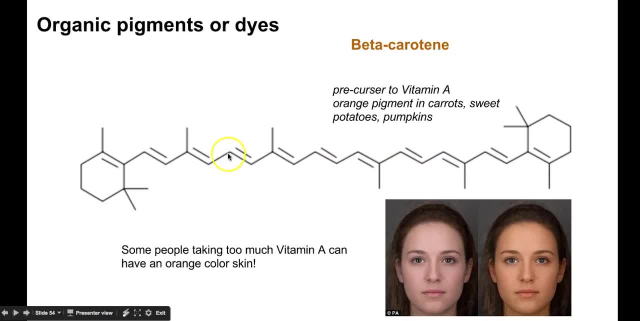 The double single, double single, which really means what? SP2, SP2, SP2, trigonal planar SP2.. That means all of these electrons are in the same energy level And you stack them all okay, Make small gaps, okay. 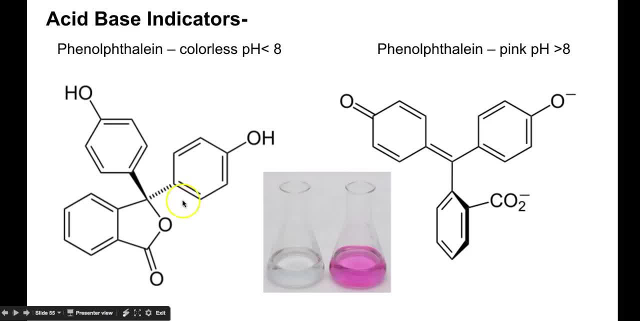 Our acid-base indicators change colors based on changing the gaps. Notice, phenolphthalein is colorless. Yes, there's like a benzene ring here and here, but they're not connected, okay, in this pH here. okay. When a pH is acidic, it changes the structure. 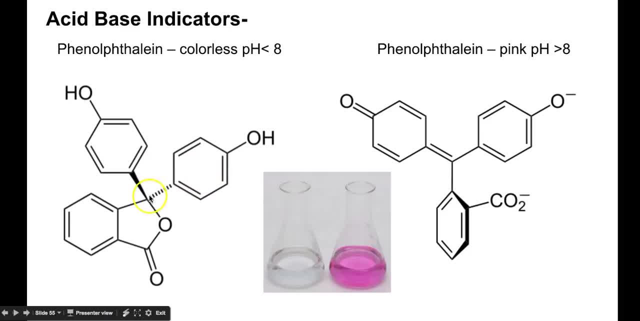 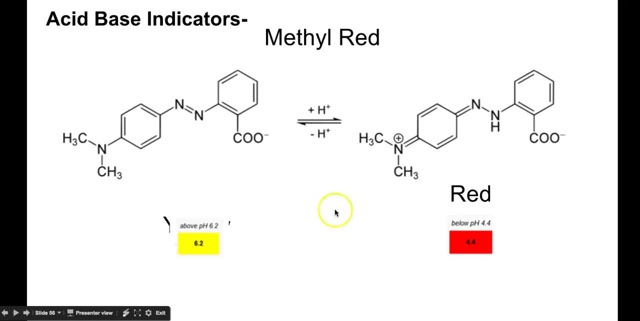 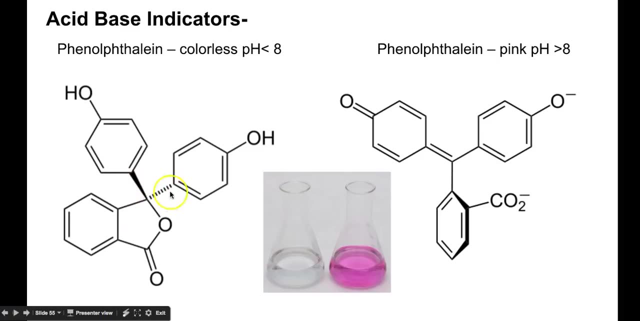 So these gaps or these electrons here are not connected. And think what happens In a basic pH: the structure changes so that now, oh my gosh, we're interconnected throughout. That is so cool. So phenolphthalein turns color because it changes its structure in different pHs to allow for more. what? 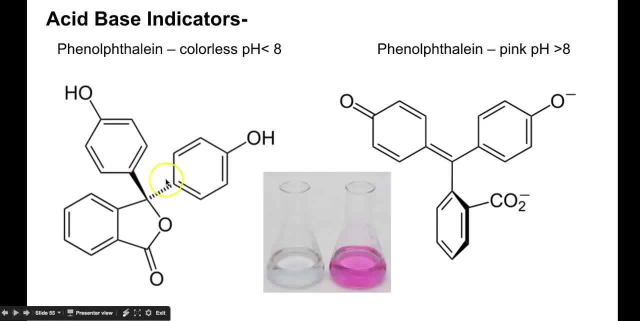 Conjugation. There's gaps here, but these gaps are too big because they're not interconnected By being at a pH of 8. Now you're connecting entire molecules, electrons, and there's more what Pi stacking here in the bonding orbitals to make a bigger continuum and smaller gap to get wavelengths of light. 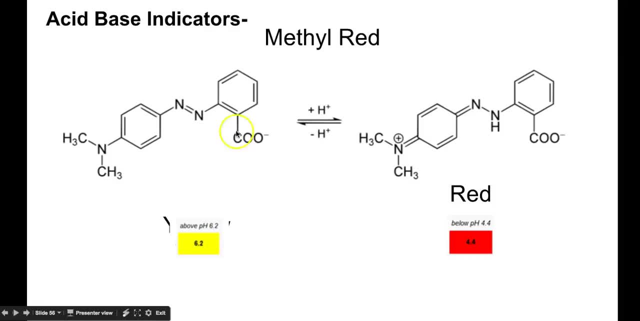 I find that to me fascinating. okay, So all of our acid-base indicators change their way of conjugation, or pi stacking, in their MO diagrams to be able to take more or less of the wavelengths of light, depending upon the gaps. The gap is changing. 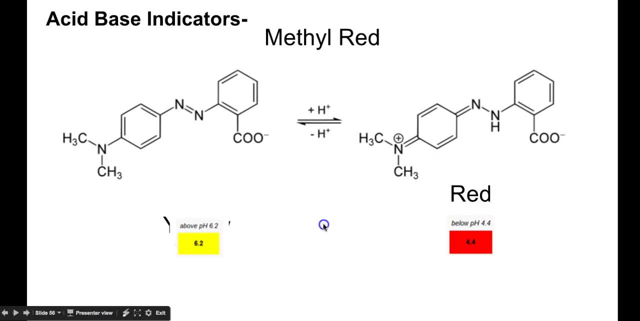 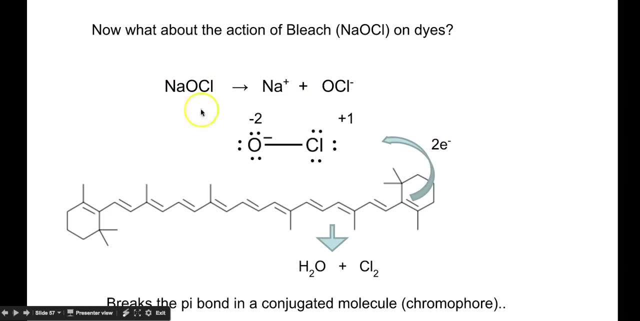 Based upon acid and base or pH of the solution they're in. And, of course, someone asked me this question a long, long time ago. Why does bleach sodium hypochlorite make our clothes lose their color? Well, sodium hypochlorite breaks apart into Na plus and the hypochlorite ion. 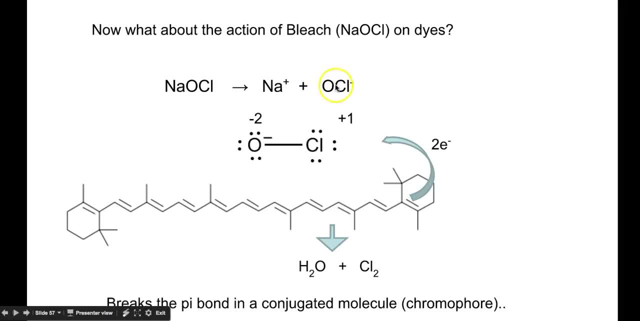 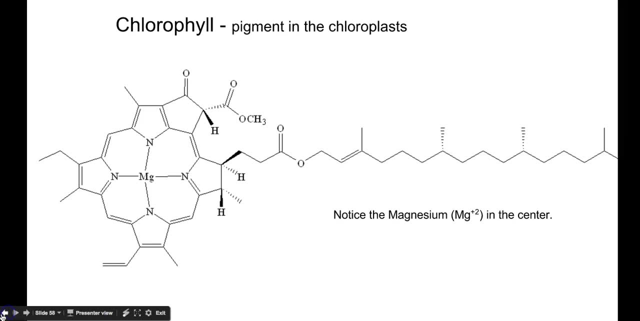 This is negative 2. This is plus 1 ion. This is a. what Electron sink And what electrons are they going to pull from Christmas in July They're going to pull from. They're going to pull from the pi bonds first because they're outside of the what? 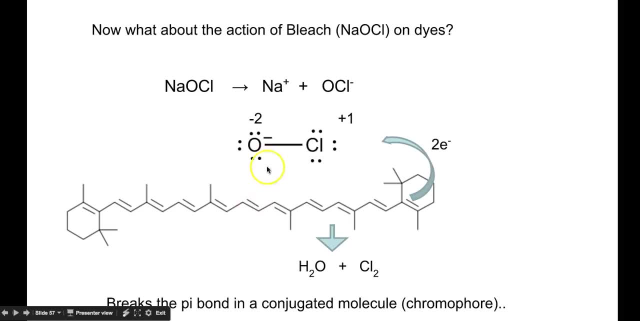 Nuclear envelope. And if you pull electrons in the middle of this beta carotene or any kind of dye and you break up the conjugation so they're not interconnected, you're going to make that continuum smaller. Keep doing that, all right. 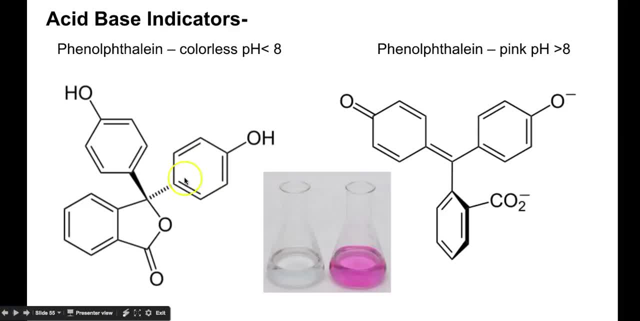 Just like we go back to phenolphthalein. There's a continuum, a band, But it's too small, Until you interconnect them so that all of these are sharing the same space. that's when the continuum gets big enough and the gaps get small enough. 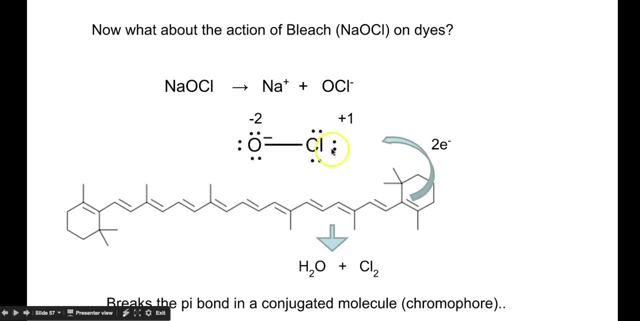 So if you drop this oxidizing agent which pulls electrons, makes this lose electrons from the pi bonds and now make this single bonds, these electrons here cannot connect. here And now the continuum gets smaller and the gap gets bigger. Hope you can understand that. 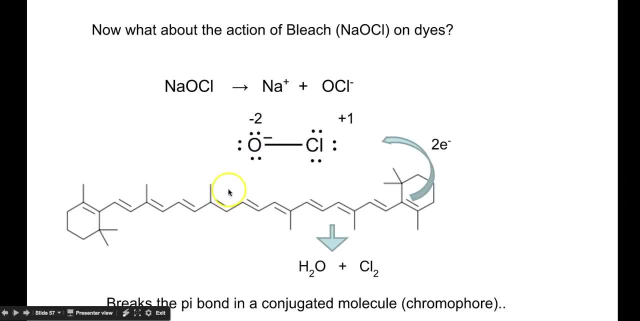 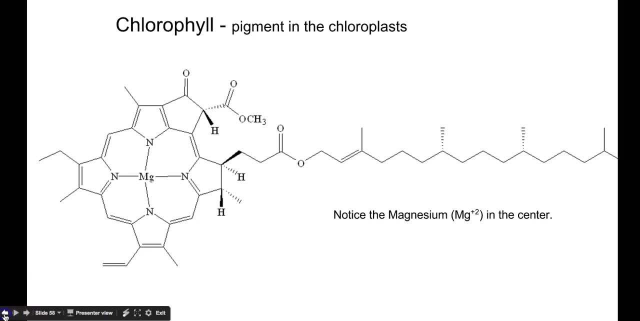 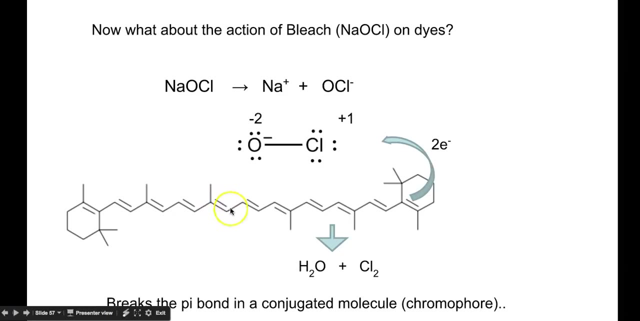 So you should know why, walking out of this, why- bleach takes our color, By the way, okay- cosmic rays and sunlight makes our clothes that have these pigments become what Become lighter over time. because we lose the electrons from the what We lose the electrons from our pi bonds. first,